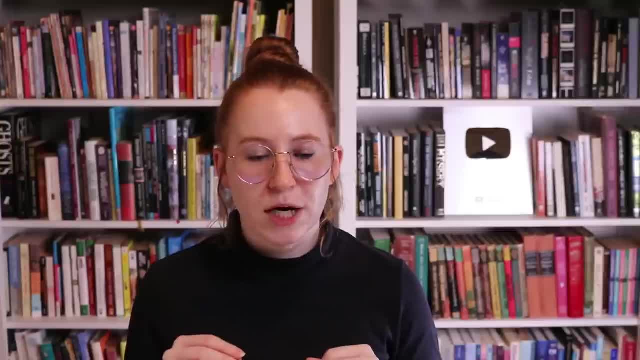 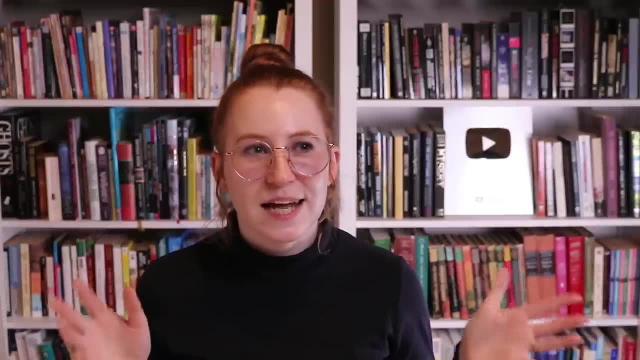 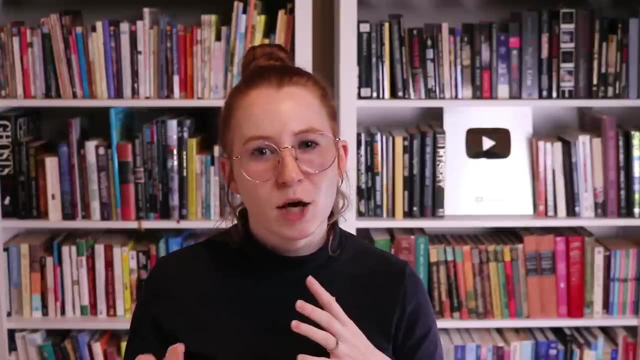 or too often it actually slows down the reading process because the reader has to try a lot harder to understand the meaning of that sentence, what you're trying to say, how it's relevant, and that can make the writing itself feel too slow And it can also make the actions feel more distant, because 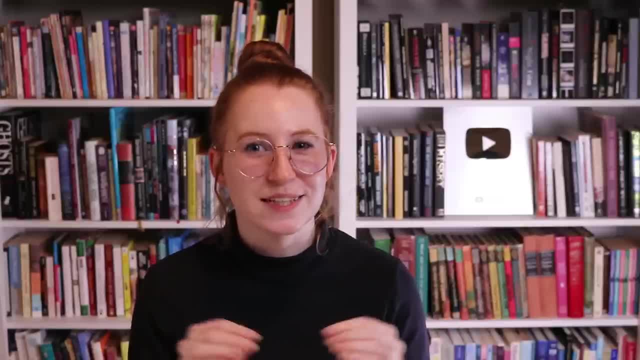 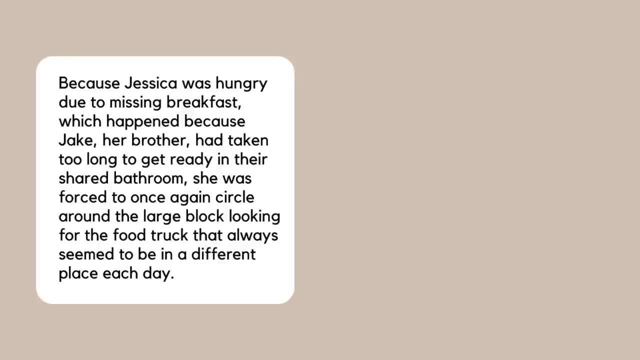 you start to layer complex sentences, So if you're writing a sentence that's too long, you might want to add more concepts and cram concepts into the same sentence. I'm going to give an example to hopefully clarify what I mean. Because Jessica was hungry due to missing breakfast, which happened because 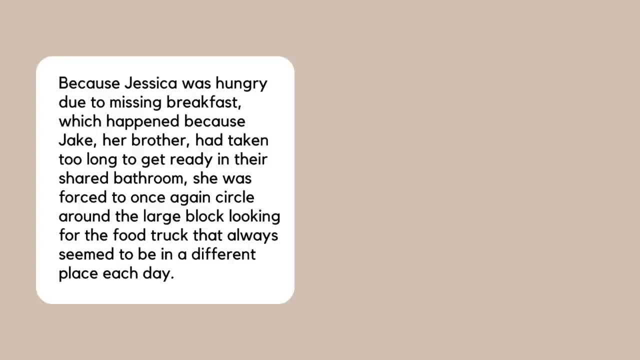 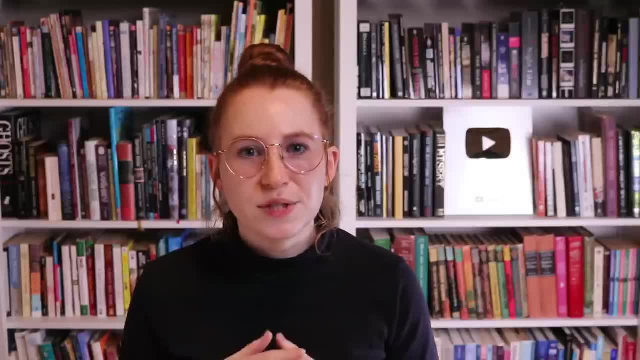 Jake, her brother, had taken too long to get ready in their shared bedroom. she was forced to once again circle around the large block looking for the food truck that always seemed to be in a different place each day. So this sentence is grammatically correct. It's pretty understandable. 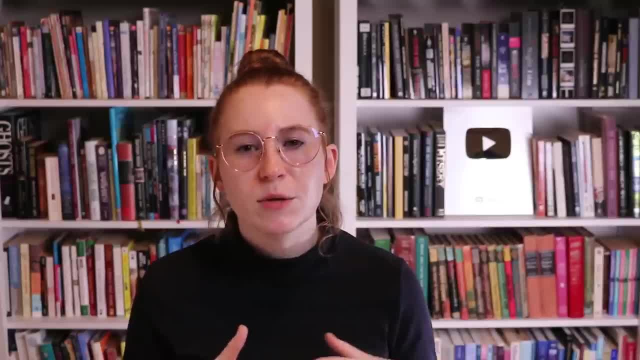 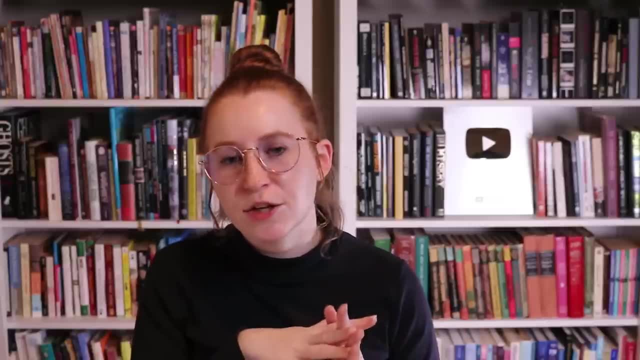 In isolation it doesn't really pose any particular problem. But if you were to take a sentence like this and combine it with several other lengthy, complicated sentences, either right up against each other or even just many times on a page or in a chapter, it will really slow down the process of. 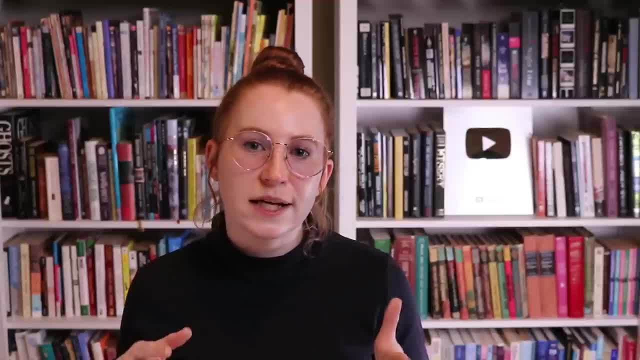 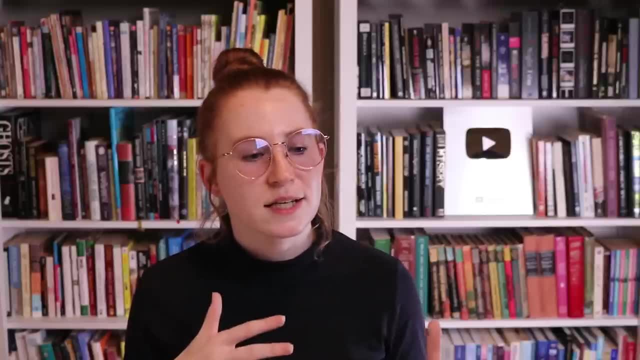 reading, The reader will have to spend longer understanding what you're saying. It may bury the point you're trying to make and it may also create distance from the action. So normally complicated sentences like this are better off broken up into smaller sentences, For example: 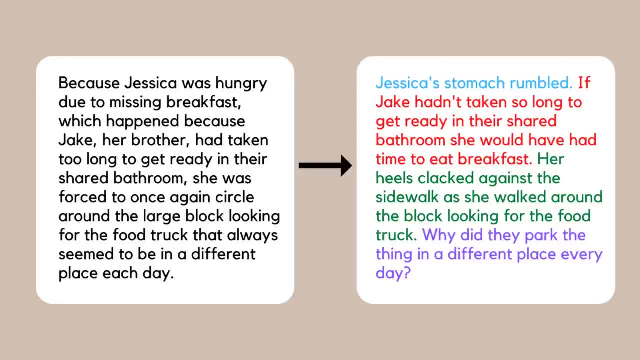 we could rewrite this sentence. If Jake hadn't taken so long to get ready in their shared bathroom, she would have had time to eat breakfast. Her heels clacked against the sidewalk as she walked around the block looking for the food truck. Why did they park the thing in a different place every day? Notice how breaking. 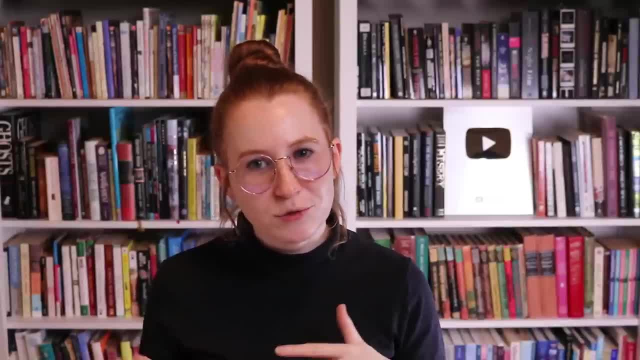 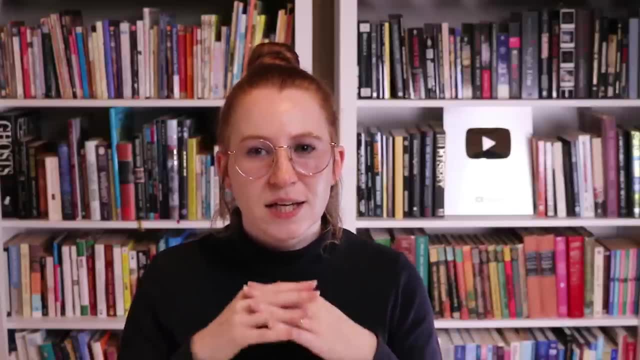 up this sentence as a bonus also gives us more room for sensory details, for some personality and introspection, and it really helps to create a more immersive experience for the reader If you have trouble identifying when sentences are getting kind of complicated or lengthy. 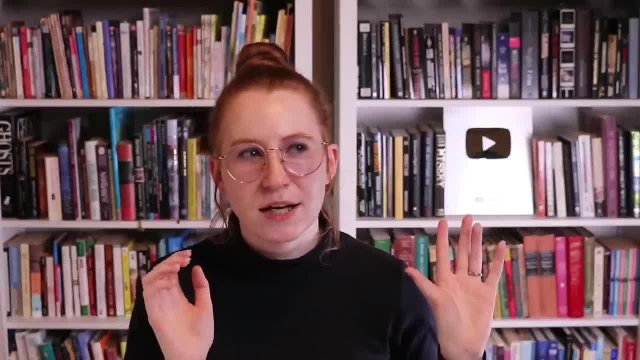 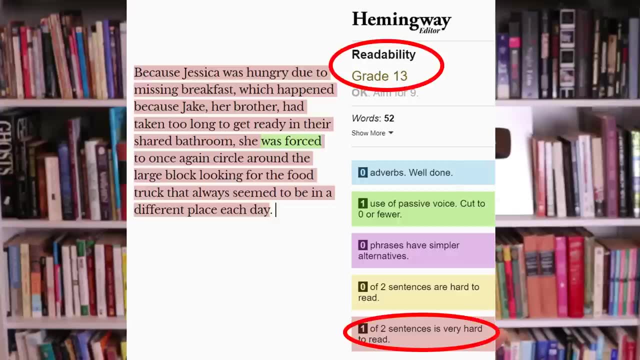 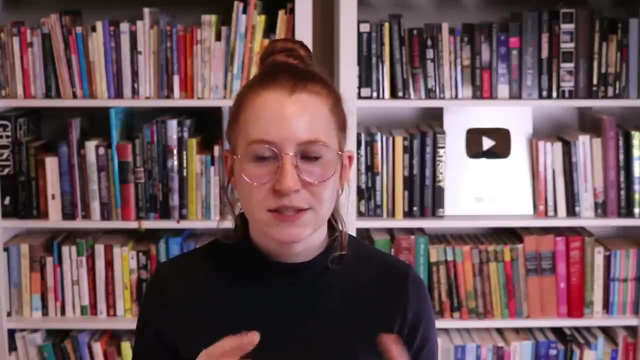 someone on my desk would say: If you put this sentence into the Hemingway editor, it has no problem identifying that the original version is very hard to read and that the edited version is easy to read. So that's something that you could use if you do struggle to tell when a sentence is getting too complicated And the 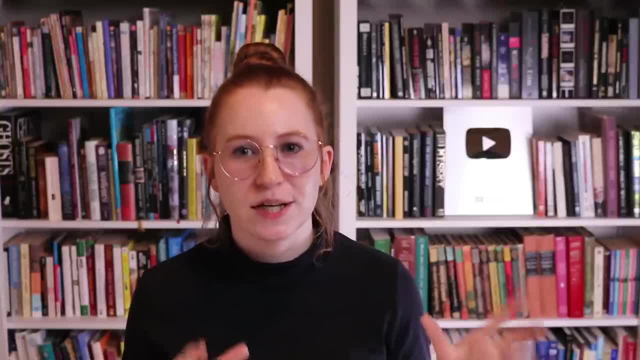 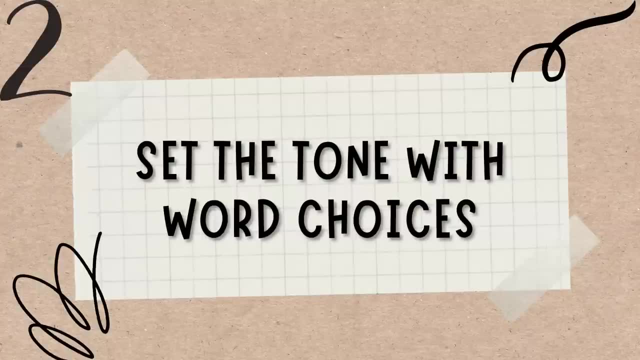 Hemingway editor actually can help with several of the things that we're going to talk about in this video, So that's just a little tip that might help you. Number two: set the tone with word choices. Often when we're writing, we can choose from a variety of words that mean basically the same. 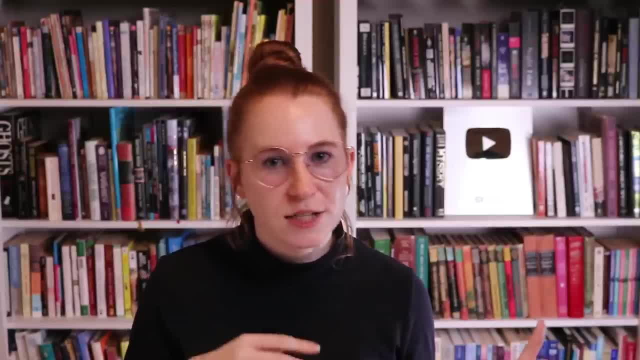 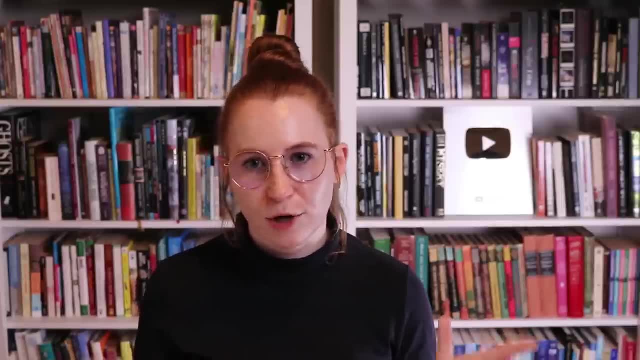 thing as what we're trying to say. But different words have very different connotations, evoke different kinds of moods, And by choosing the right word you can really improve the overall tone and vibe of your writing. For example, the boat sliced through the water feels aggressive. 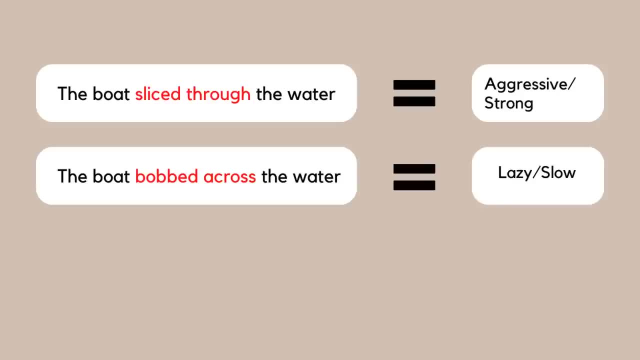 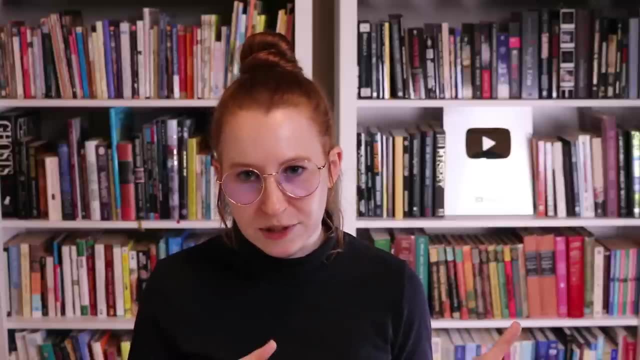 or strong. The boat bobbed across the water feels lazy or slow. The boat floated over the water might feel hopeful or even uplifting. This also goes for similes. If you're writing a romantic scene, you don't want to describe the roses like blood spots on the bed. 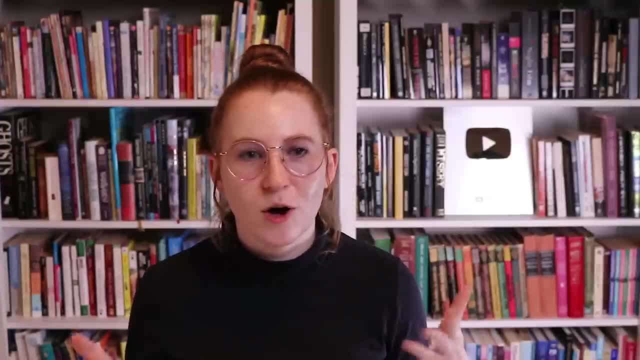 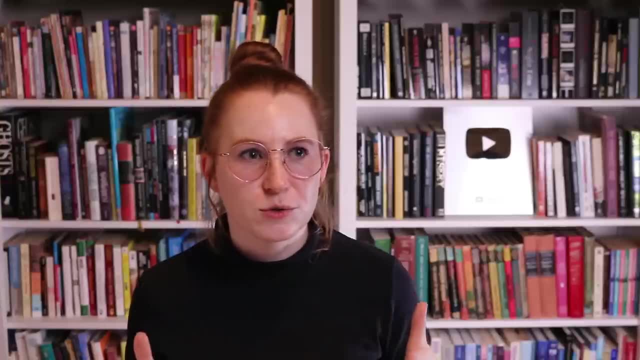 And if you're writing a horror, you don't want to describe the long hallway as a giraffe's neck, because it just doesn't set the right mood and tone. So be thoughtful about the words that you're choosing and the impact that's having on the vibe that you're writing is creating. Let's look at an 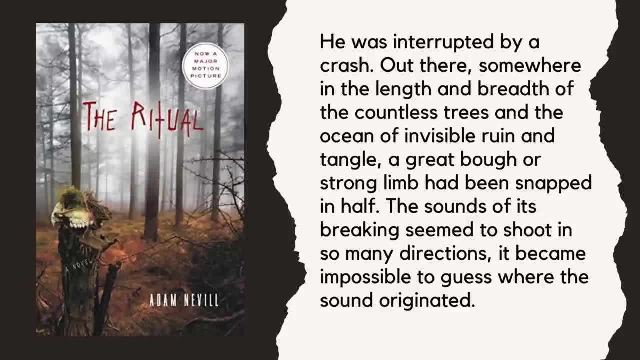 example from the novel The Ritual by Adam Neville. This is, of course, a horror novel, and pay attention to the words that he chooses. He was interrupted by a crash. Out there, somewhere, in the length and breadth of the countless trees, in the ocean of invisible ruin and tangle, a great bough or strong limb had been snapped in half. 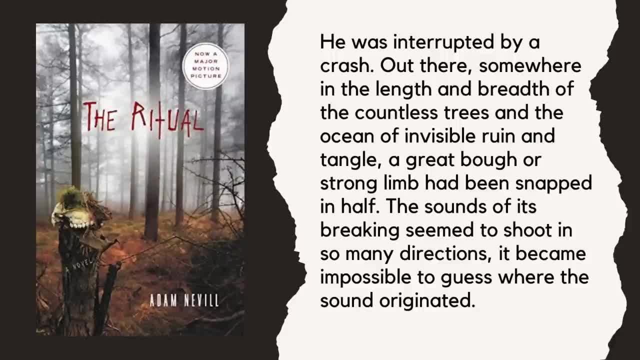 The sounds of its breaking seemed to shoot in so many directions it became impossible to guess where the sound originated. Notice how the word choices emphasize the largeness of the woods with the ocean of invisible ruin and tangle. Also notice the emphasis on more aggressive sounding. 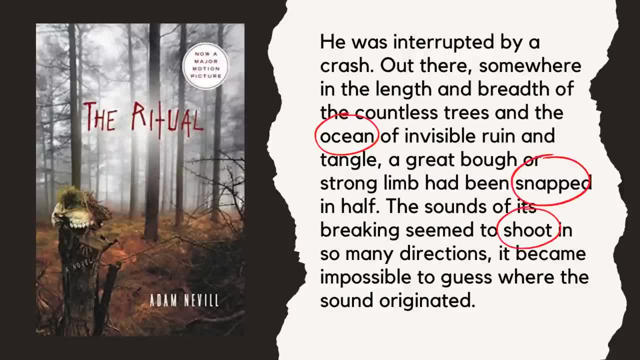 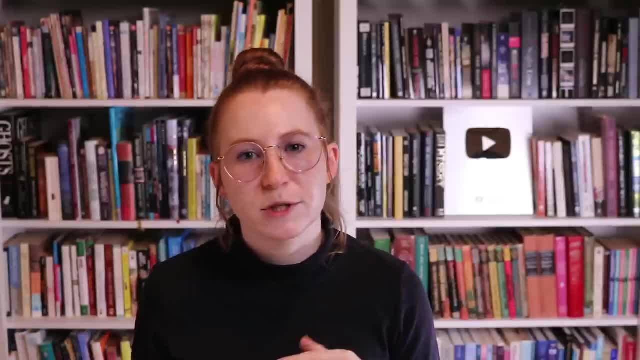 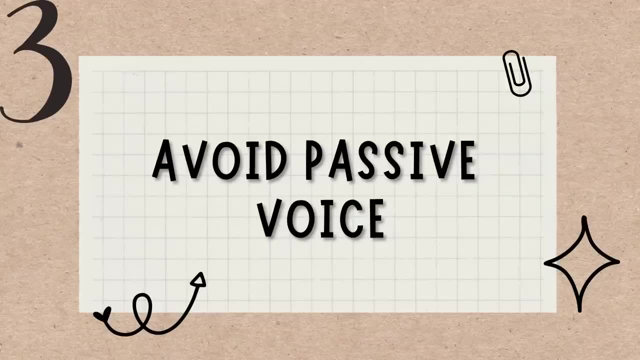 words like snapped in half rather than broke, and the sound shoots in so many directions. Try to create the mood or the vibe that you want the reader to experience with your word choices, and this will really go a long way towards improving your writing. Number three: avoid passive voice. You've probably heard a million times that you should avoid. 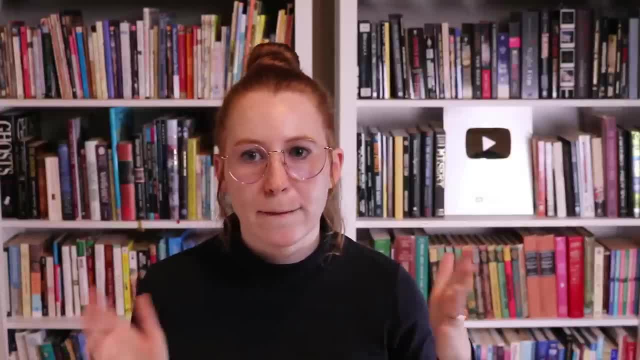 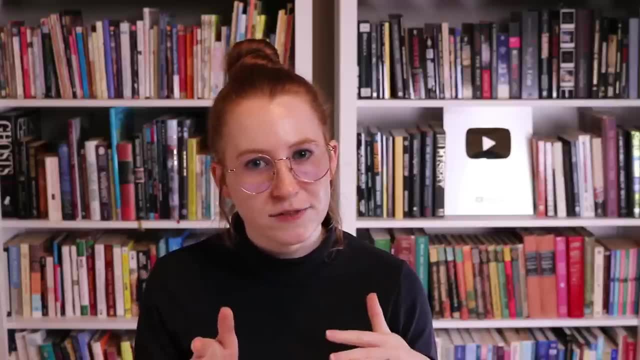 passive voice. Sometimes it can be a little tricky to understand what that means, but to make it as simple as possible, passive voice is when the subject of a sentence or the clause of a sentence perceives the action instead of performs the action. So if you're struggling to tell, 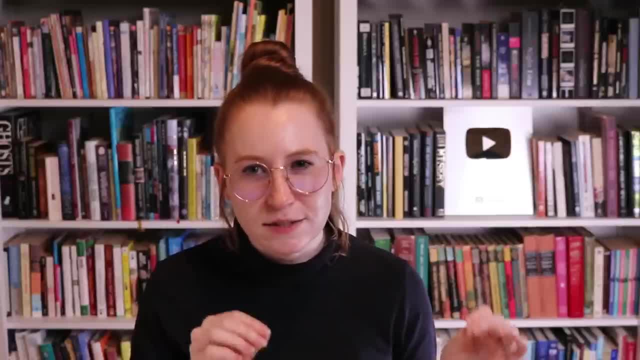 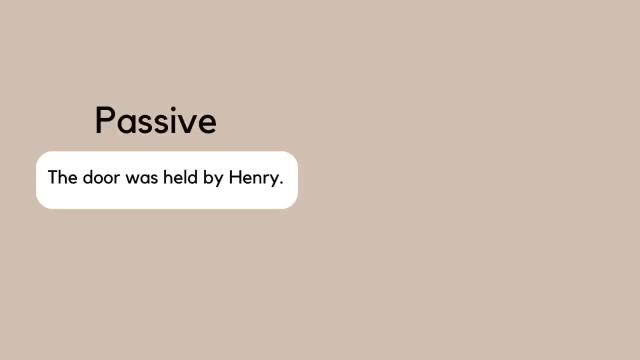 is this passive voice? is it not passive voice? just try to ask yourself: is the subject doing the action? Are they performing the action? For example, the door was held by Henry is passive because the door is not doing the action, whereas Henry held the door is active. Henry is the one. 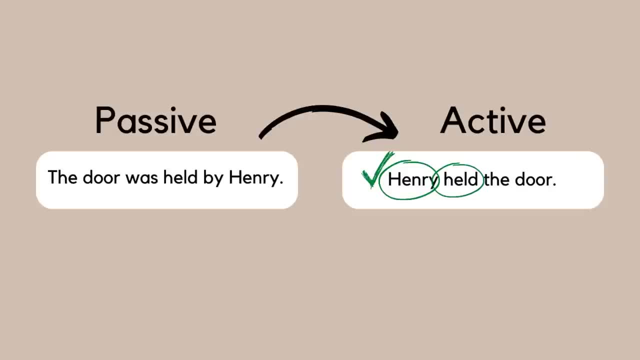 doing the action of holding the door. Often in fiction this can be a problem because it results in de-emphasizing the character doing the action. Here's another example: In the first sentence, Meghan was chased by Elizabeth. is we compared to Elizabeth chased? 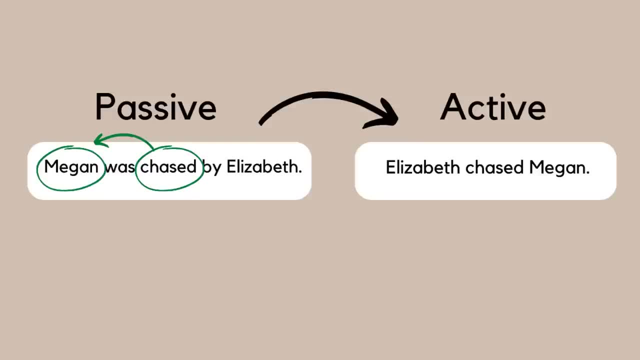 Meghan. In the first sentence, Meghan is receiving the action and in the second sentence, Elizabeth is doing the action. Even if Meghan is the protagonist- so the character we generally want to emphasize more- the writing will feel stronger if we focus on the person doing the action. 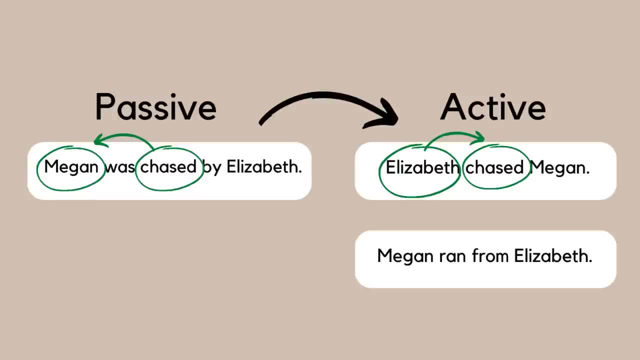 If we do want to put more emphasis on Meghan, another option might be: Meghan ran from Elizabeth, so we want to put more emphasis on Meghan to still be the one who's actually doing the action. So we're still not using passive voice. There may, of course, be situations where we want to use 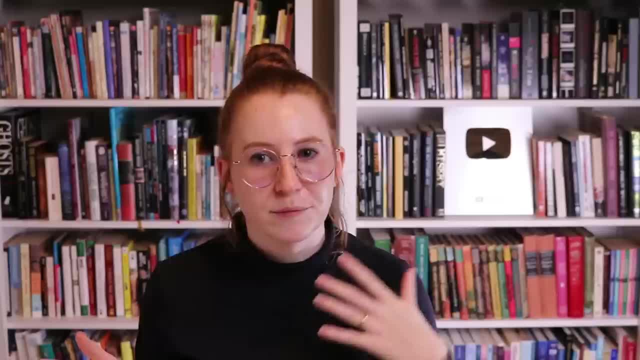 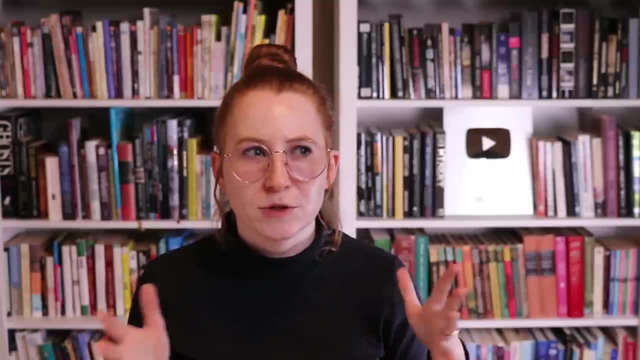 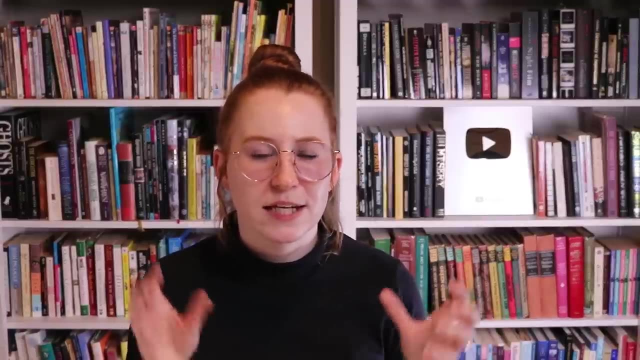 passive voice on purpose to create a certain effect, such as intentionally creating distance. A character might do this for some reason, such as not wanting to take responsibility or maybe feeling guilty. So in deep third POV or in first person POV, it's possible that passive 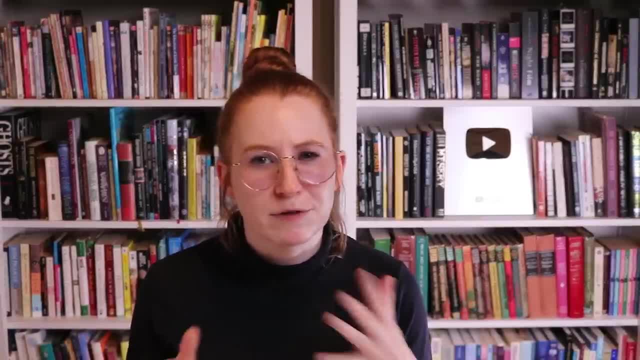 voice might help to convey that intentional distancing from the action, But I would say that if you're using passive voice, you might want to put more emphasis on the person doing the action. So if you're using passive voice, you might want to put more emphasis on the person doing the action. 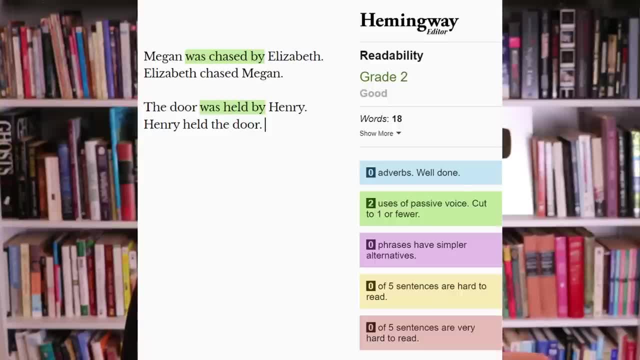 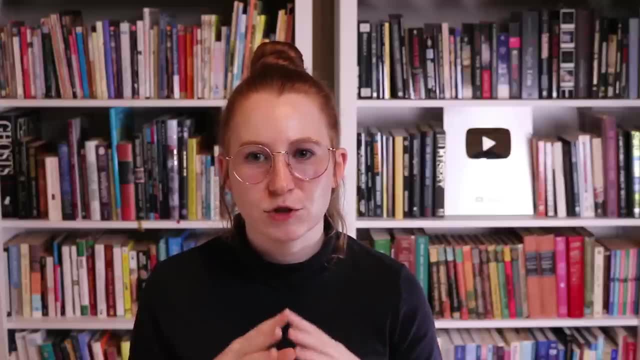 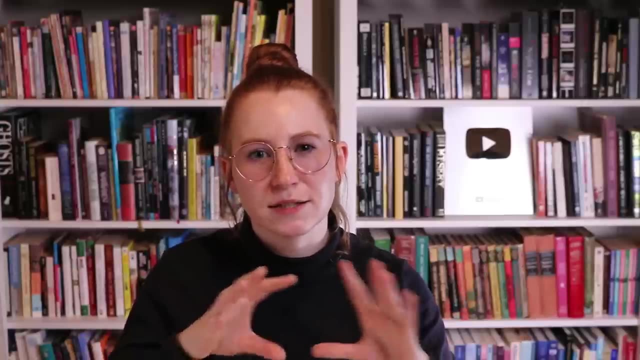 Again, the Hemingway editor can really help with that. It does a pretty good job of identifying passive voice. Number four: remove filtering. So filtering is when the experience of the story is filtered through the POV character, So that character's experience is emphasized as separate from the reader. That's not really what. 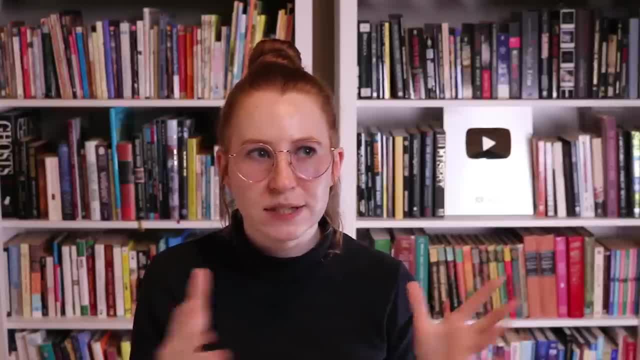 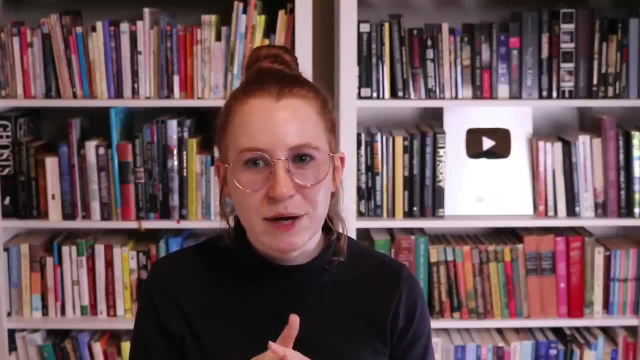 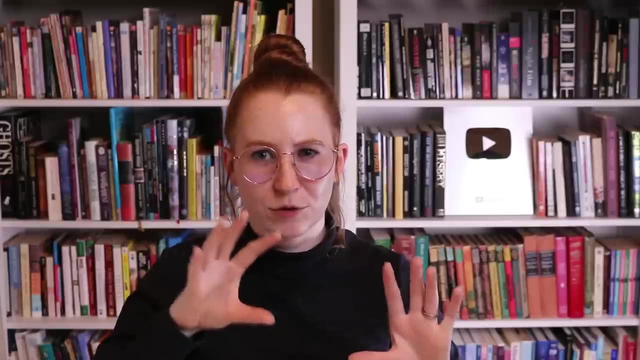 the intention is. That's what the effect of filtering is. Filtering typically involves using words like thought, knew, felt, saw, smelled, tasted, things that create a separation from the sensory experience and the reader. I'm going to give examples because I 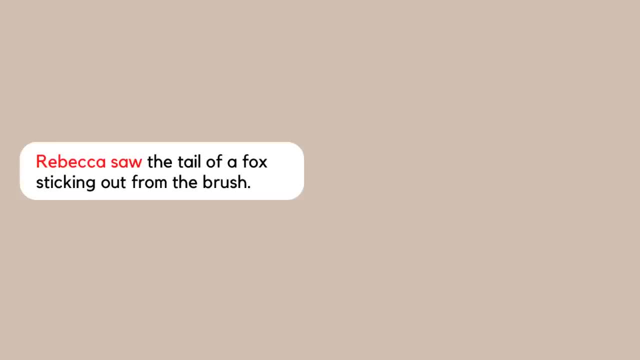 think that makes this a lot easier to understand. A common filtering word in amateur fiction is saw. So, for example, Rebecca saw the tail of a fox sticking out from the brush. It's more distancing than the tail of a fox stuck out from the brush. 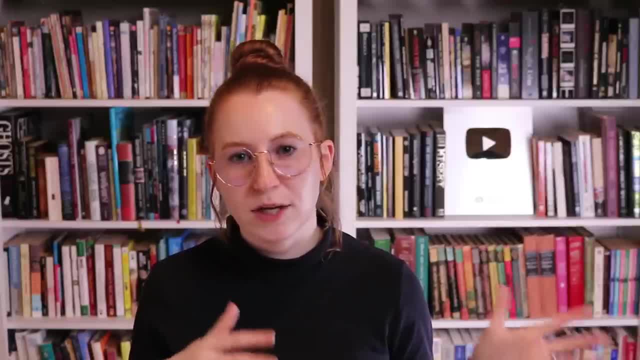 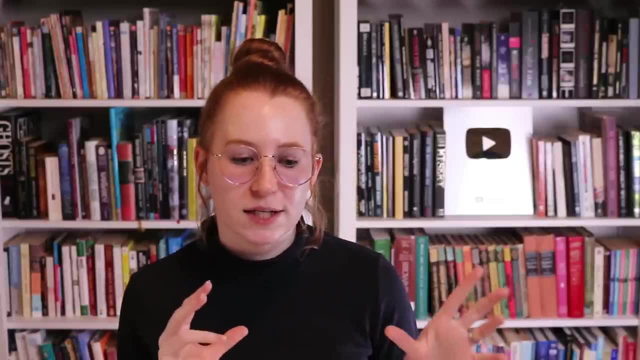 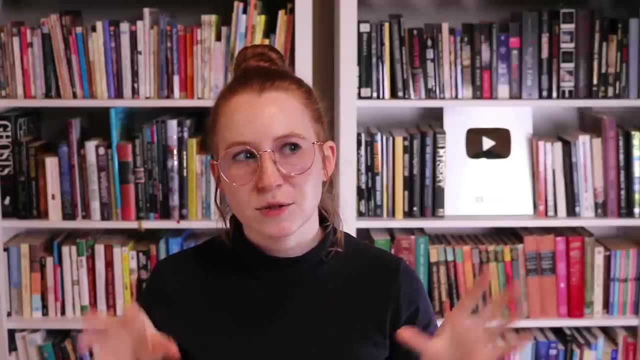 Of course there are sensory words where there isn't really any way to work around them, For example, smelled and tasted. It's not really easy or feasible to try to write a sentence where you describe that without using the words smelled or tasted, But we can still create a slightly more. 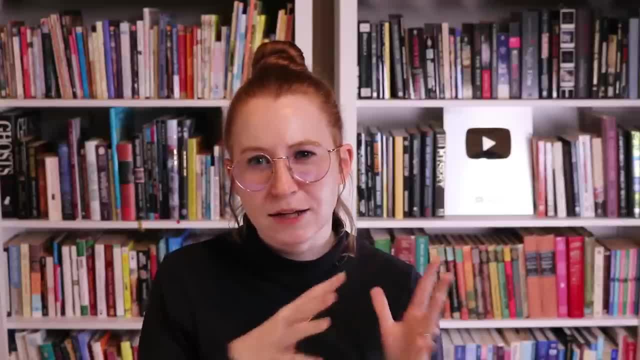 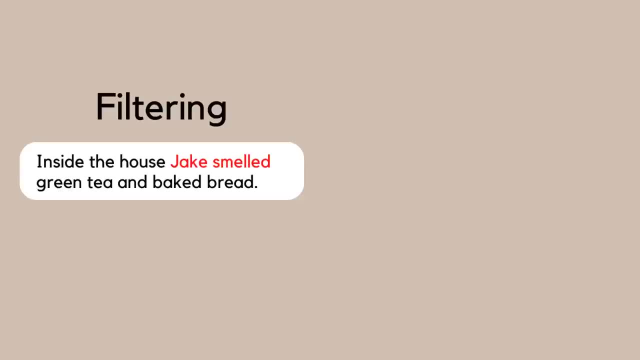 immersive effect by again eliminating filtering that through the POV character. For example, inside the house, Jake smelled green tea and baked bread. It could be easily made stronger by rewriting it as the house smelled of green tea and baked bread, which eliminates that distance between the sensory experience and the reader. 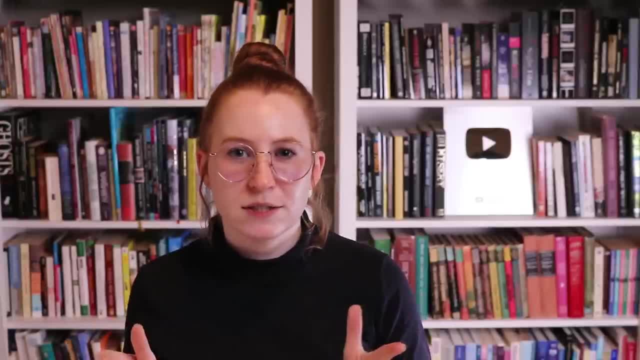 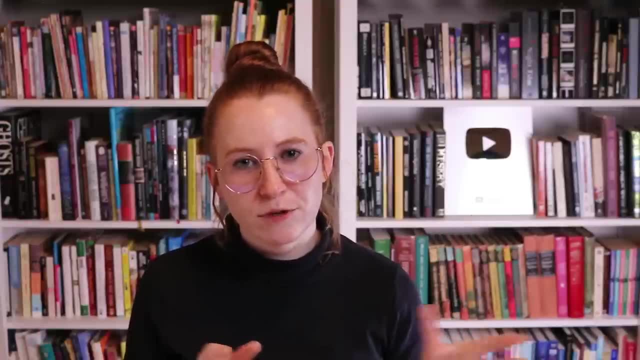 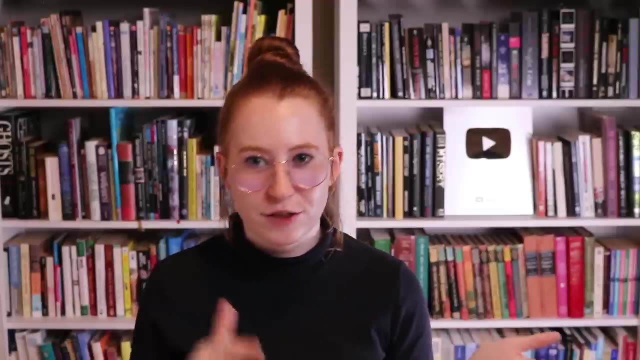 Introspection can also be less impactful and more distancing when we use filtering like knew, wondered, thought things along those lines. So whenever we're using a deep point of view or first person point of view, we can assume that it's the character, the POV character thinking the thought or having the realization. So those 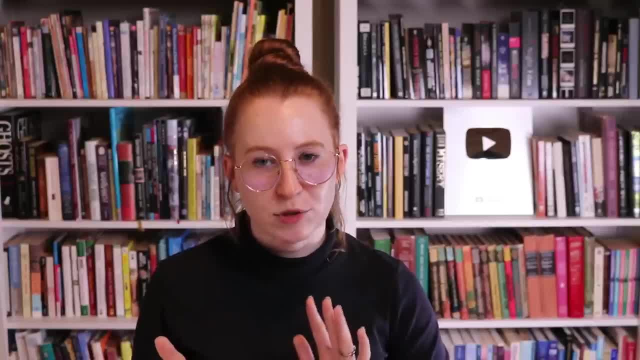 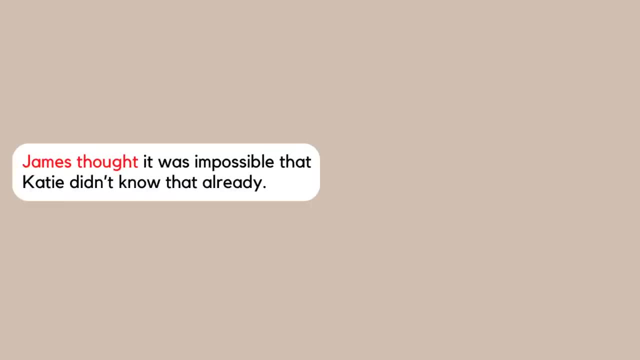 add a little bit extra and unnecessary separation between the reader and that thought, realization etc. For example, James thought it was impossible that Katie didn't know that already. It's a lot weaker than it was impossible for Katie not to know that already. 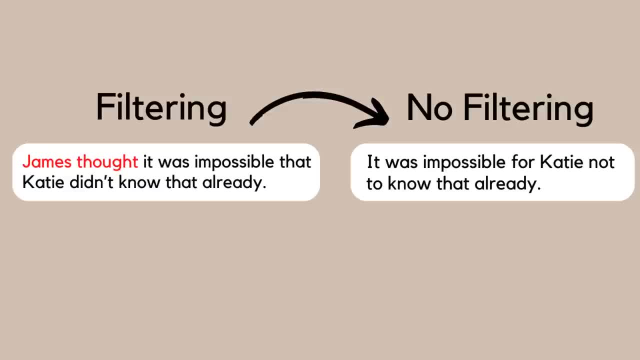 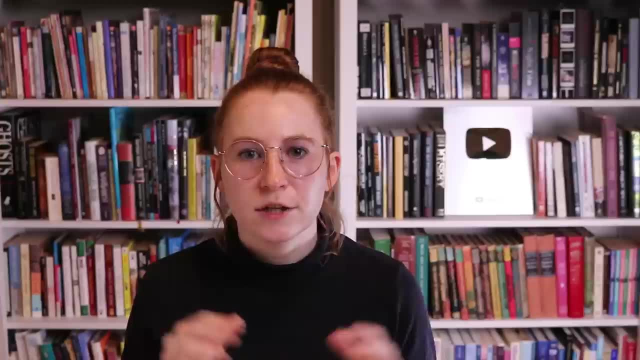 We don't need to say that James thought it was impossible, because James is the POV character, so we can simply say it was impossible and it doesn't make the writing feel quite as distant. Of course, there are times where filtering might help with clarity. 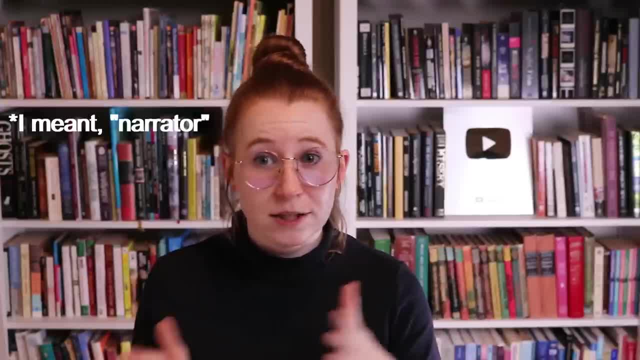 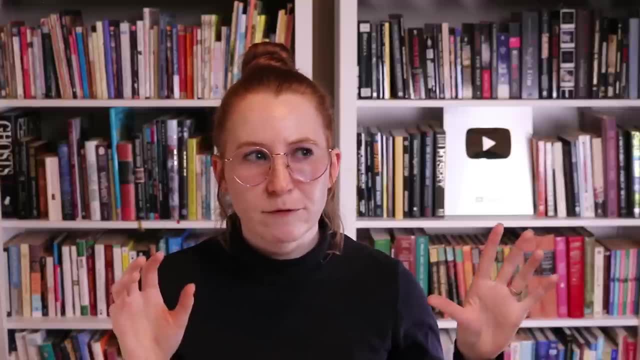 such as an omniscient point of view, where there's a difference between what the character knows and experiences versus what the characters know and experience. So in that case filtering might help with clarity. But for most writers today, the majority are writing in deep, third, limited or first person. 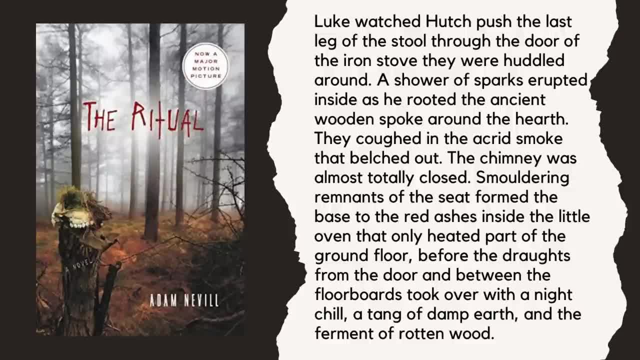 and in neither of those cases is filtering really beneficial. Let's look at an example from The Ritual. At the beginning of this excerpt, it's pointed out that a character is watching something, which is a form of filtering. However, in this case, the character 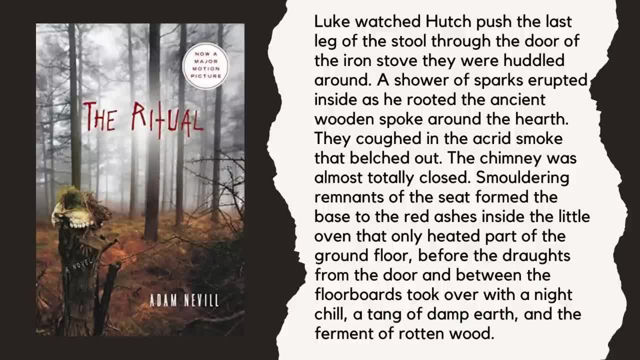 is exhausted and inactive, so it may be intended to put emphasis on this inaction by saying that he watched what's occurring. But note how the rest of the paragraph has no filtering and a lot of sensory details. In that excerpt we get a lot of sensory information: sights and smells. 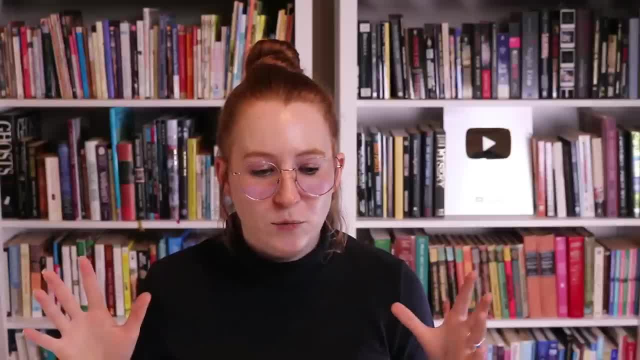 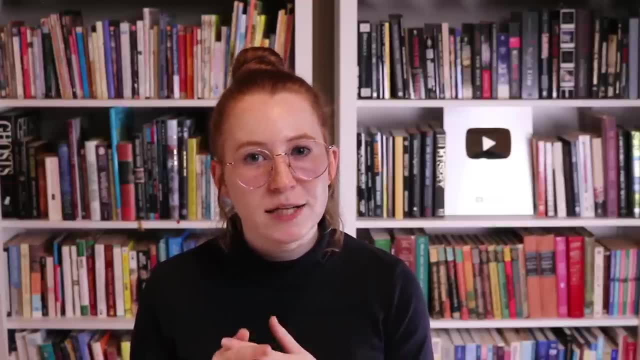 even a little bit of taste, maybe of the smoke, And we did not need to use filtering words to bring that across. So it's a much more immersive experience for the reader. So, if possible, eliminating filtering is a great way to make the reading experience feel a lot more. 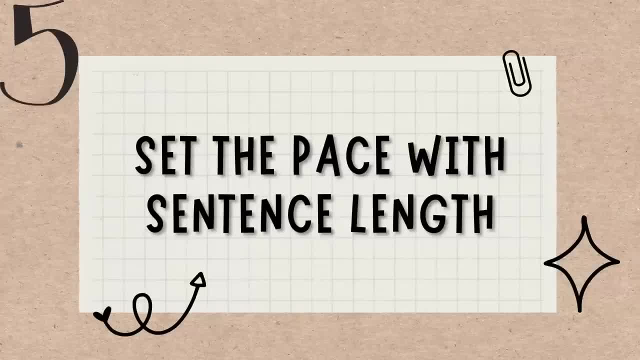 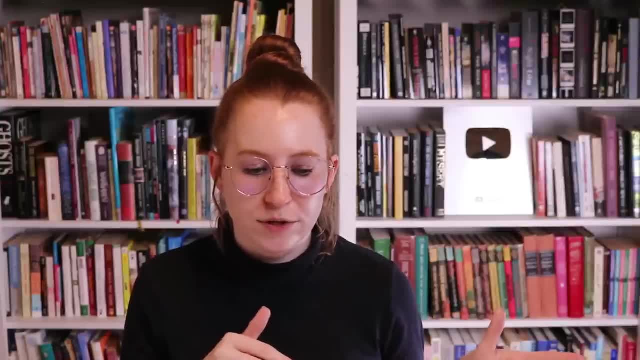 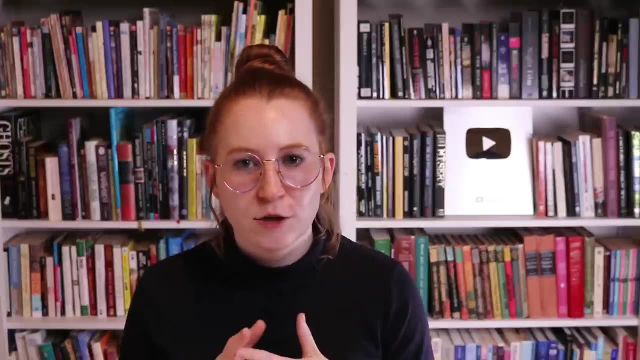 immediate, a lot more connected to the reader. Number five: set the pace with sentence length. It's not only word choices that can help with setting the tone or the mood. The sentence length can also go a long way towards setting the tone or mood of a scene. For example, in most cases, 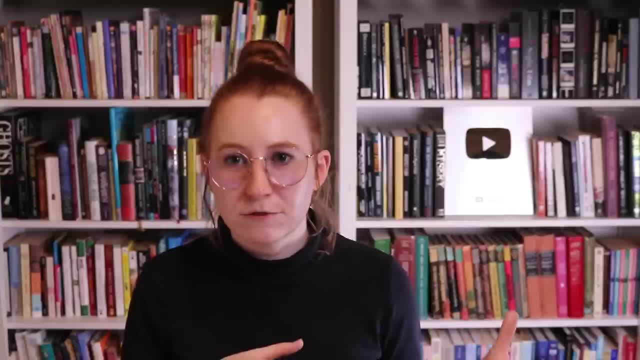 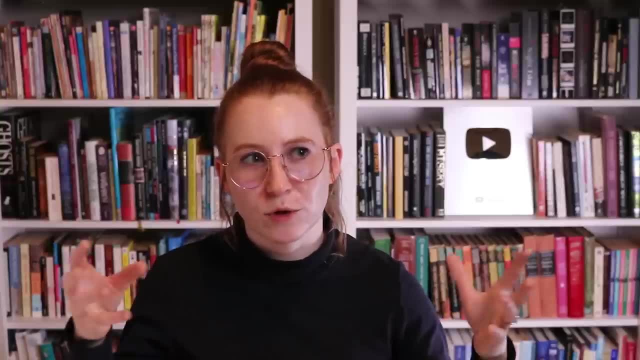 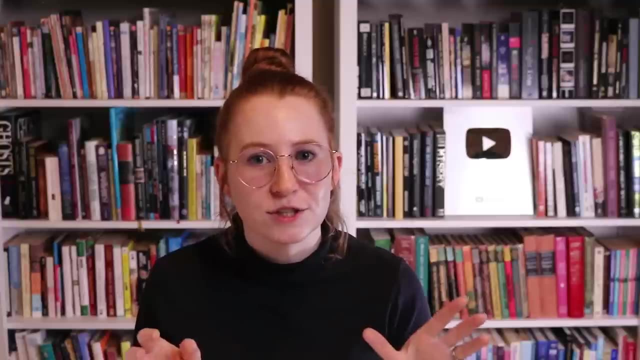 if the character is being thoughtful, or maybe they're distant from something that occurred, longer sentences tend to work better. They give a more introspective, thoughtful mood, Whereas if the character is involved in an intense or immediate emotional situation, action, urgency, all of that is better conveyed by shorter, choppier sentences. This is a really 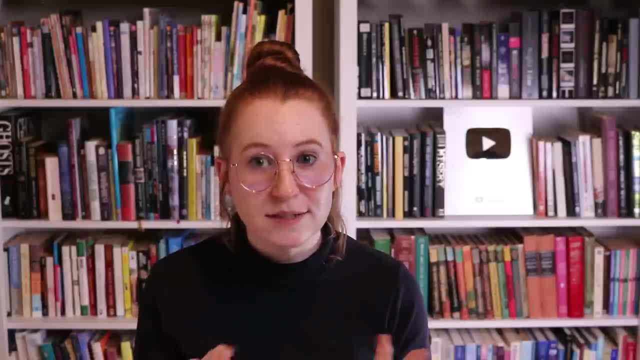 great way to control the pace that the reader reads. So when we have shorter, choppier sentences, we tend to read faster and that can help to give a sense of tension and urgency, Whereas when you want to give that more more creative, thoughtful, introspective type vibe, maybe the character is 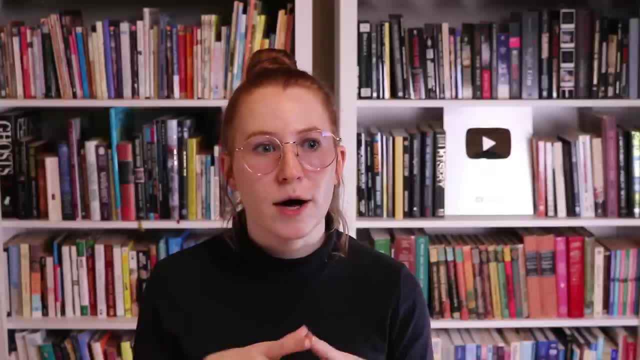 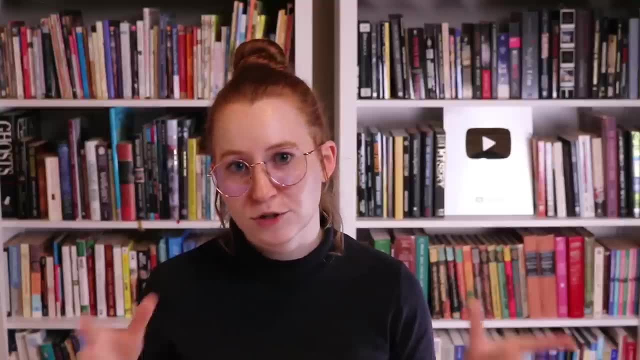 observing things, or maybe they're just watching a movie or they're just reading a book, So that's, They're thinking about the way things look. the descriptions, visual descriptions, sensory descriptions- Those things tend to work better in longer form, with longer sentences, slower reading. 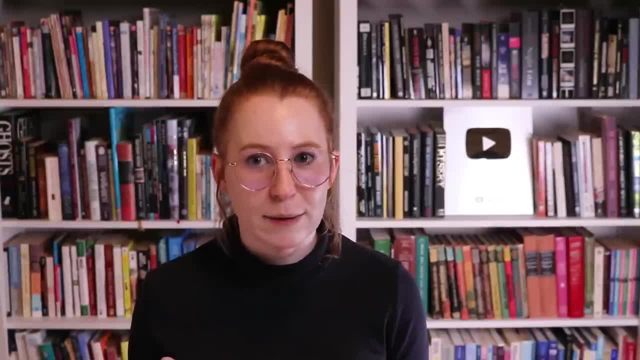 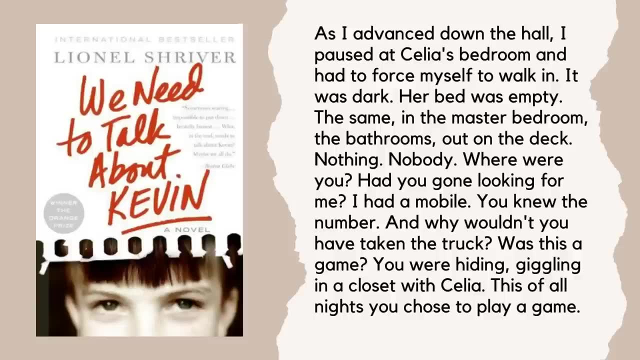 time more of a experiential vibe. Let's look at two examples from the same book. So we're going to look at. We Need to Talk About Kevin by Lionel Shriver. Notice in this intense scene where the protagonist comes home to a concerningly quiet house. 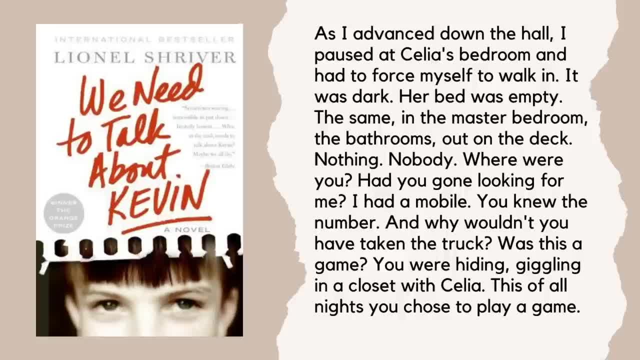 how short the sentences are. As I advanced down the hall, I paused at Celia's bedroom and had to force myself to walk in. It was dark. Her bed was empty. The same in the master bedroom, the bathrooms out on the deck, nothing, nobody. 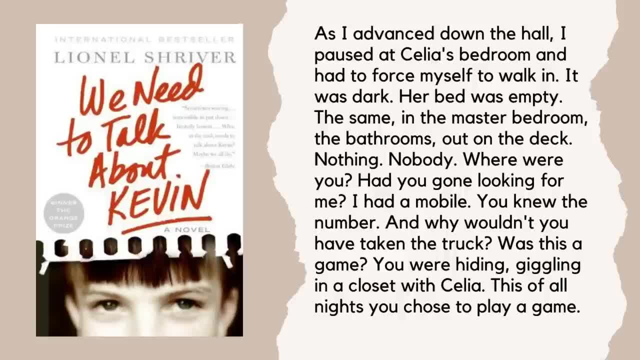 Where were you? Had you gone, looking for me? I had a mobile, You knew the number And why wouldn't you have taken the truck? Was this a game? You were hiding, giggling in a closet with Celia. This of all nights, you chose to play a game. 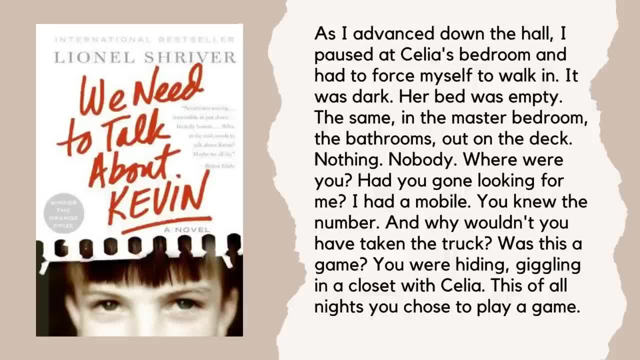 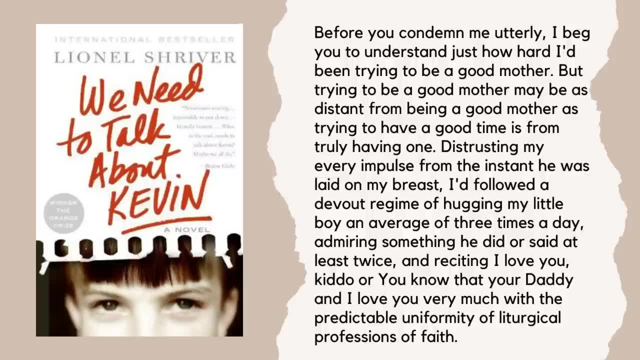 The shortness conveys her sense of panic and urgency. We can compare this to another point in the book that focuses more on reflection or thoughtfulness. Before you condemn me utterly, I beg you to understand just how hard I'd been trying to be a good mother. 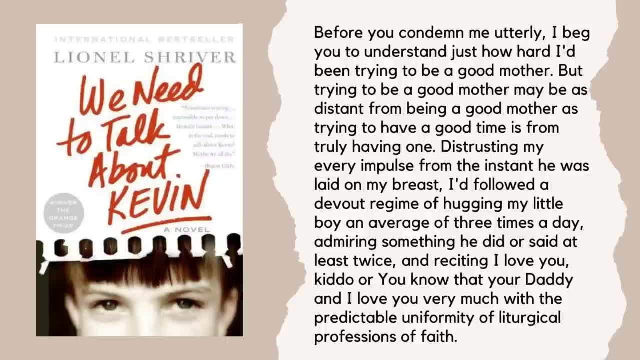 But trying to be a good mother may be as distant from being a good mother as trying to have a good time is from truly having one. Distrusting my every impulse, from the instant he was laid on my breast, I'd followed a devout regime of hugging my little boy an average of three times a day, admiring something. 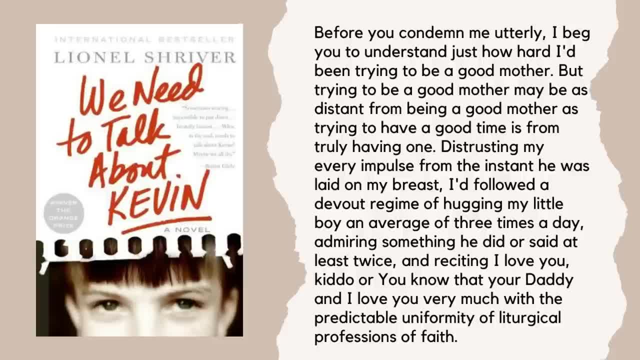 he did or said at least twice, and reciting: I love you, kiddo, or you know that your daddy and I love you very much. with the predictable uniformity of liturgical professions of faith, The longer sentences here convey a sense of thoughtfulness as well as emotional distance. 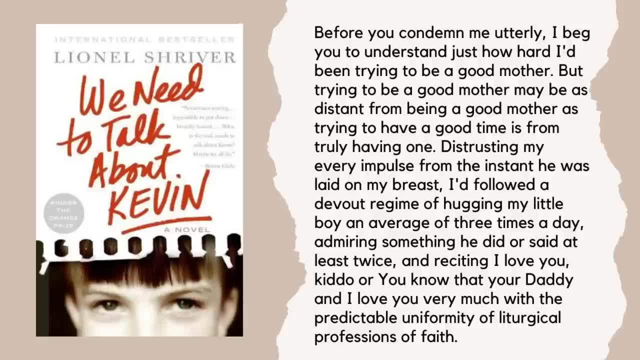 from the material being discussed. She's explaining here and wants to be understood, but there isn't an urgency and the emotions of the situation feel at least partly past. But if the sentences were shorter or choppier, it would instead come across as more desperate. 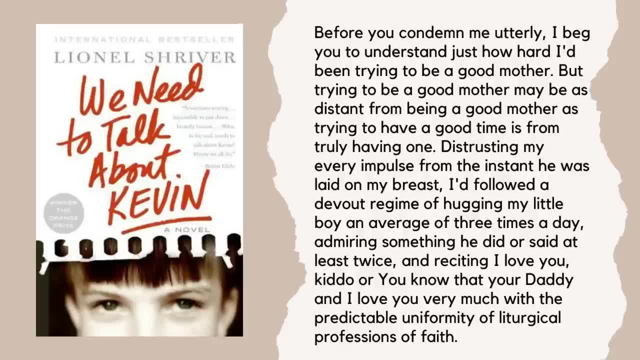 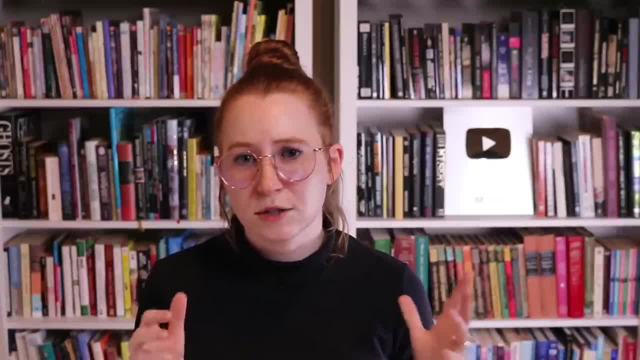 or panicked, or maybe that she has immense stake in being understood in this moment. The sentence length can vary a lot throughout the novel, even throughout individual scenes. It's a great way to control the pacing and it can really give your writing that extra edge. 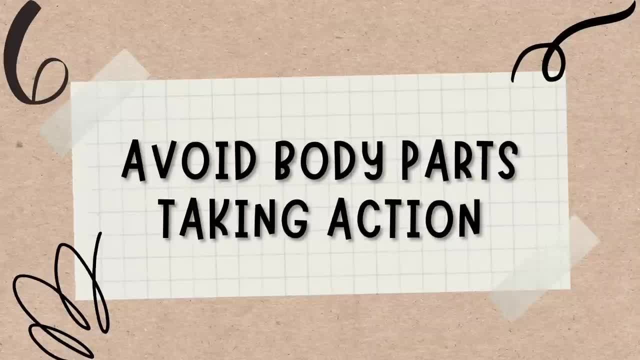 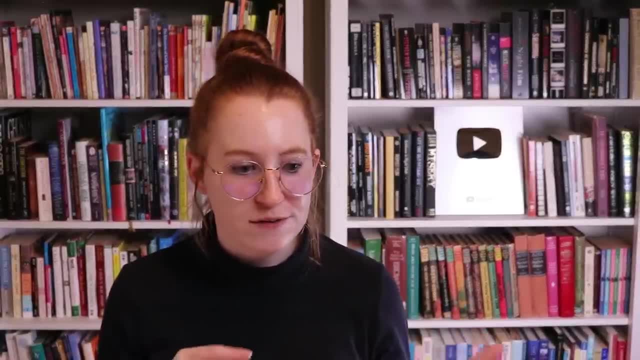 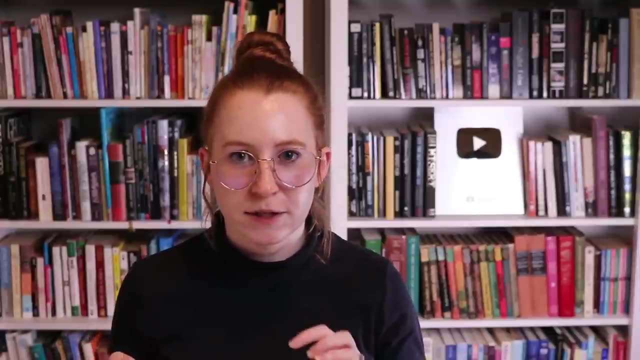 Number six: avoid body parts taking action. This is a very common habit that amateur writers can get into, but it's very easy to fix. So once you're aware of it, you can easily cut it out of your writing. So sometimes, the way sentences are written, the body part of a character is given the 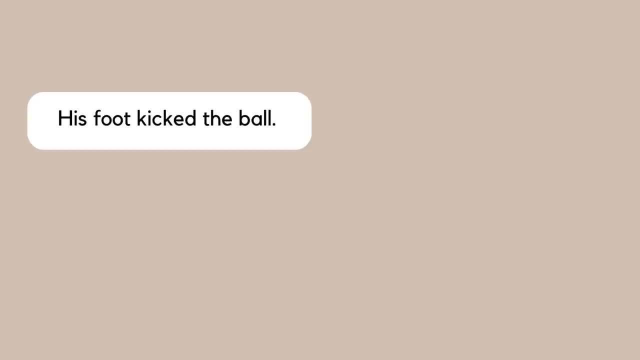 action rather than the character themselves doing the action. For example, his foot kicked the ball, The ball gives the action to the foot, while he kicked the ball gives the action to the person. Her hand grabbed. the pen gives the action to her hand, while she grabbed the pen gives. 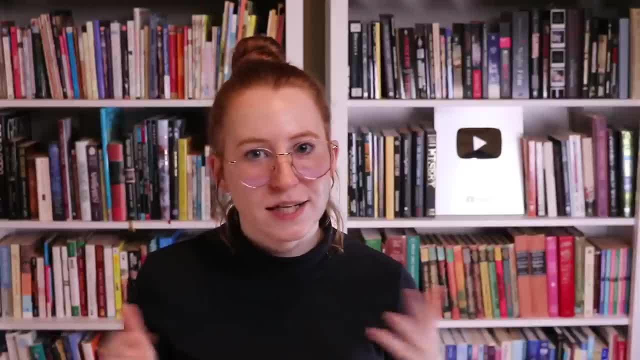 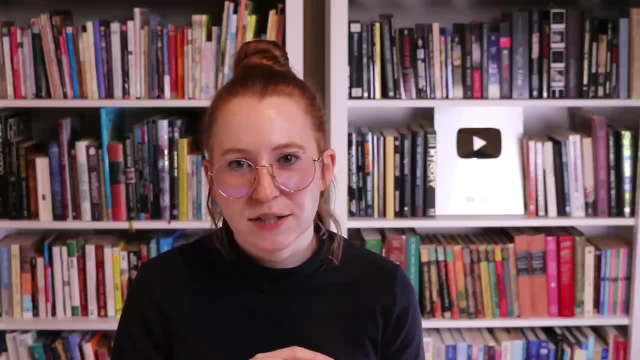 the action to the person. This again creates unnecessary distance from the action. But it's a very simple and easy to take out of your writing. But it's definitely something I recommend to give your writing a little more strength. Number seven: reduce was ING construction. 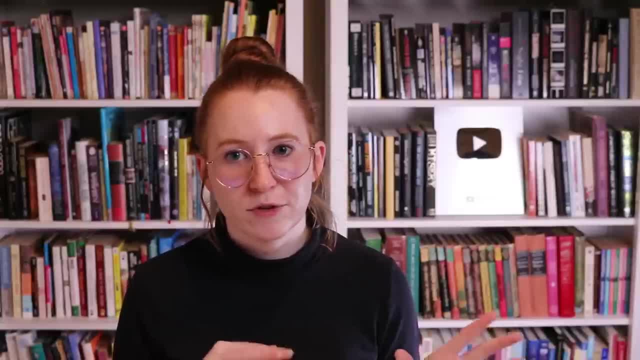 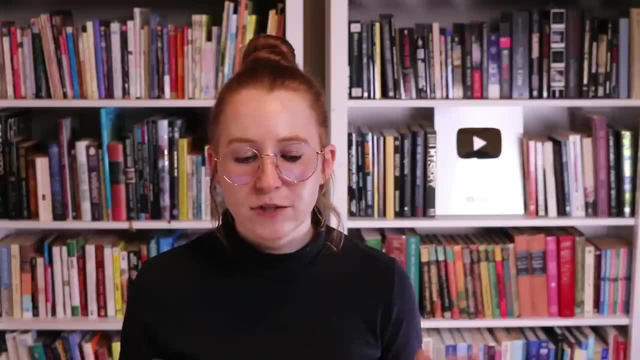 So this is another super easy one. once you're aware of it, you can easily remove it from your writing. writing and that is just that. the was ing construction. so was running, was dancing, was jumping, feels more distant from the reader and also just feels weaker. for example, he was running. 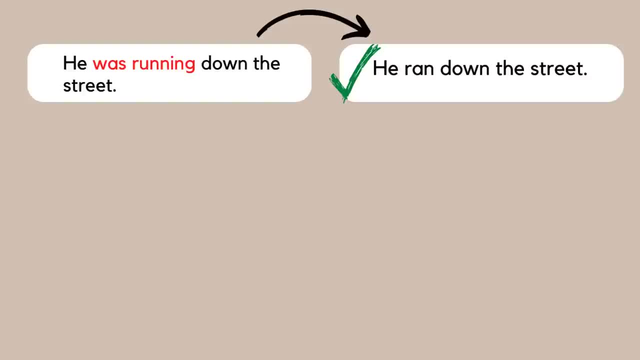 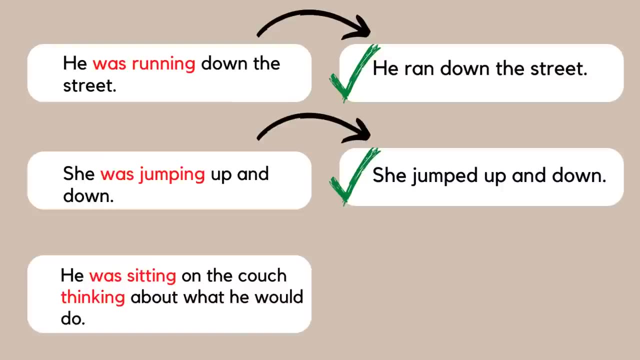 down the street could be easily made stronger by rewriting it as he ran down the street. she was jumping up and down is better as she jumped up and down. he was sitting on the couch. thinking about what he would do is not as strong as he sat on the couch and thought about what he would do. 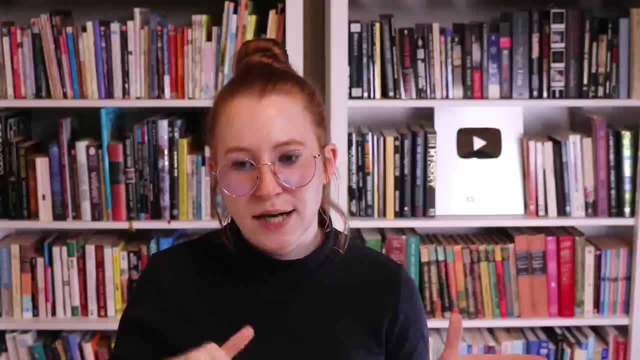 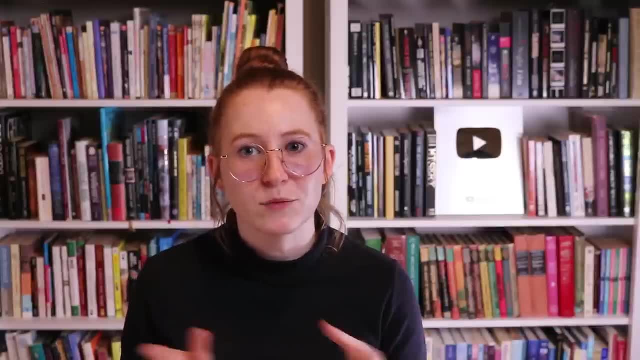 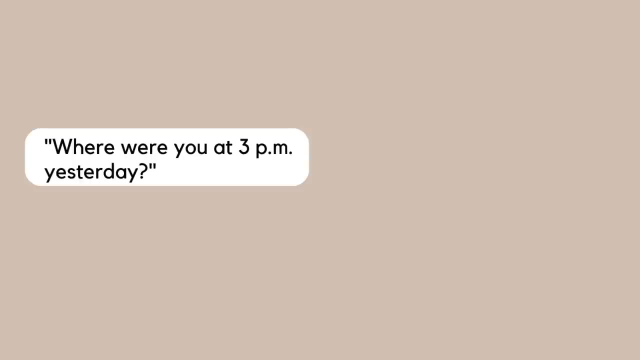 of course there might be situations where the was ing construction just sounds more natural or does convey a slightly different meaning, and in that case it's completely fine. we should always go with what sounds best and most natural. for example, in dialogue, if a character asks another character where were you at 3 pm yesterday, they will most likely respond with i was driving home. 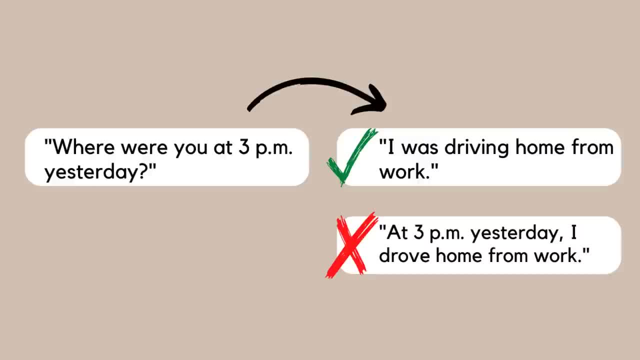 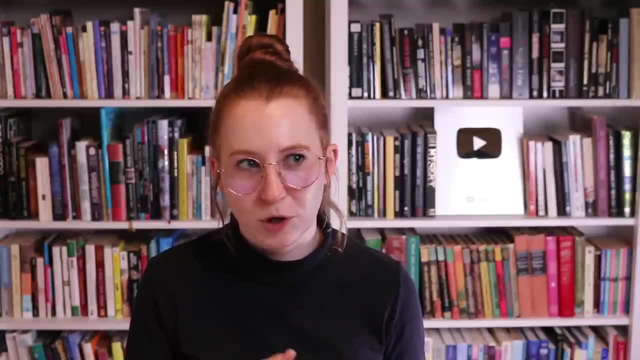 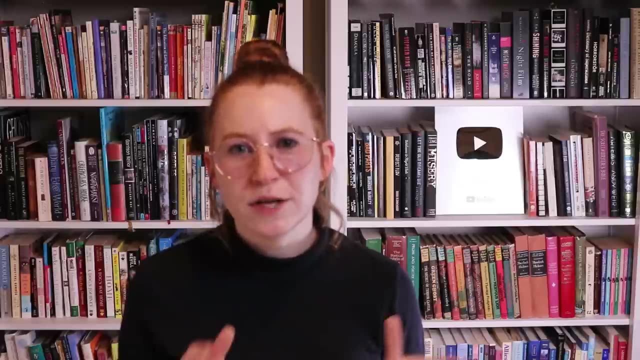 from work rather than at 3 pm. yesterday i drove home from work with all of these tips. the point is to make the writing feel stronger. so if one of these tips ever makes your writing feel more unnatural or awkward, of course don't follow it. number eight: keep the wording natural. often writers might go for more unnatural phrasing. 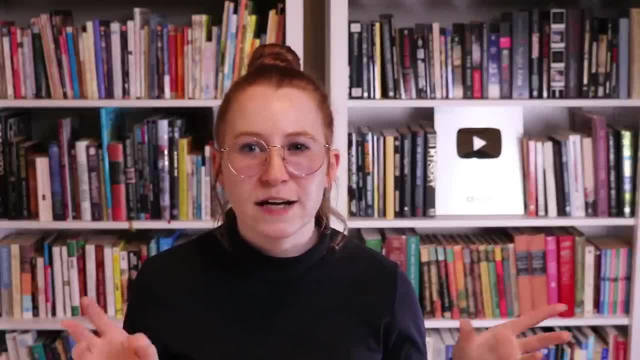 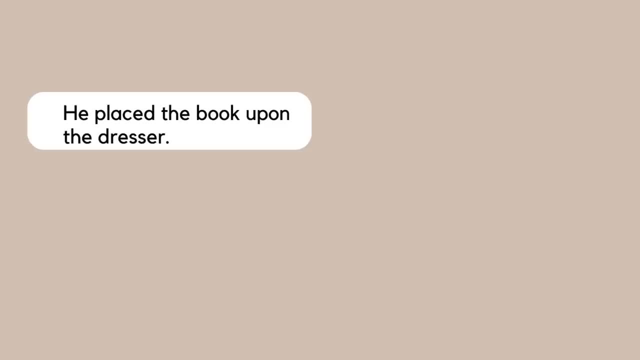 in an attempt to sound more sophisticated, old-fashioned writerly, but normally this doesn't enhance the writing. it can feel a little bit awkward or even maybe stiff. for example, he placed the book upon the dresser rather than he sat the book on the dresser. the second sentence is a lot. 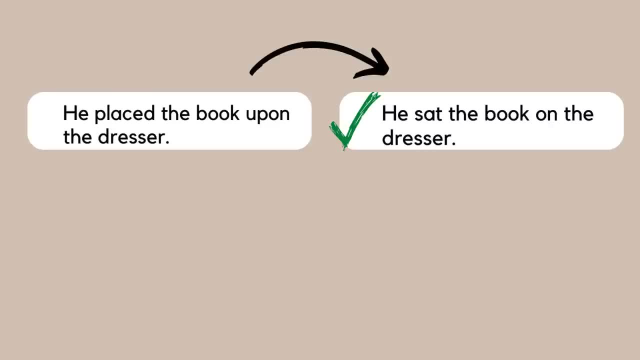 more natural. so if one of these tips ever makes your writing feel more unnatural or awkward, of course a lot more natural, a lot more how modern people would talk or explain something, the more sophisticated, old-fashioned. he placed the book upon the dresser sounds kind of awkward to modern. 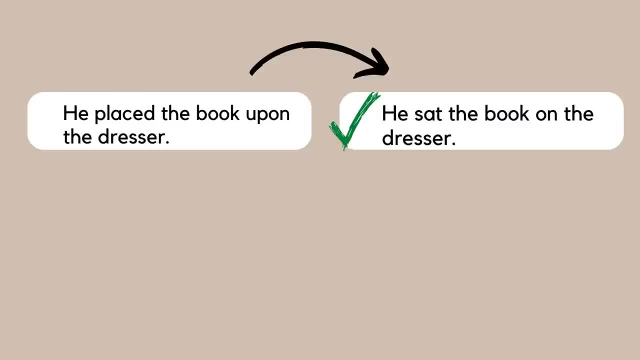 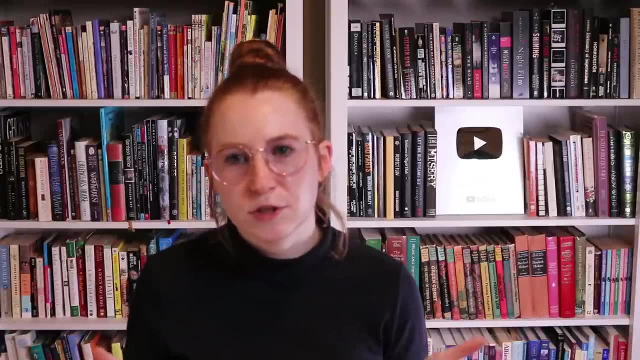 readers. sometimes this could also take the form of avoiding contractions such as writing he did not know what he should do, rather than he didn't know what to do. there might, of course, be situations where it makes sense for the personality of your character. that may be the narrator, the style of 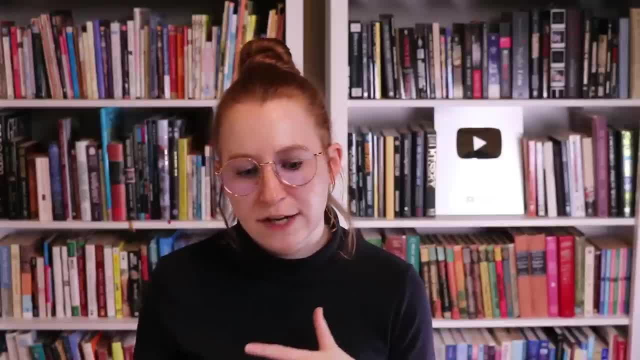 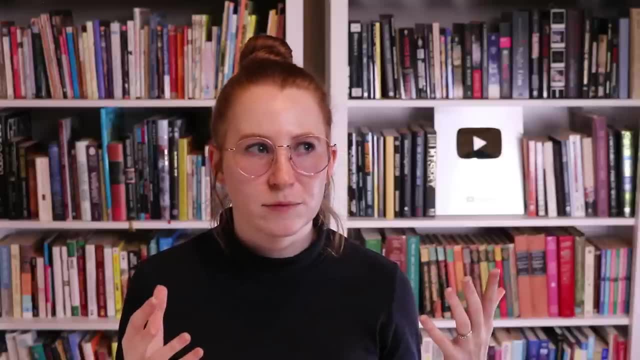 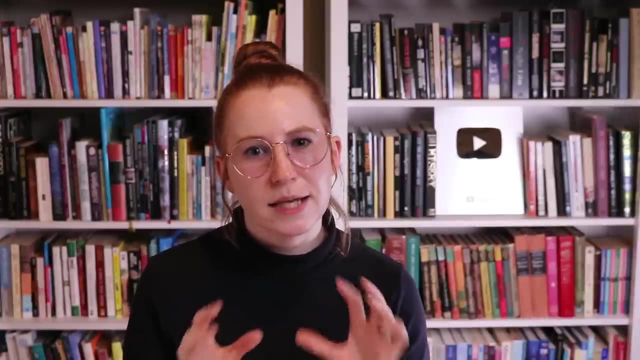 writing. there may be reasons why going for a more old-fashioned or sophisticated sound makes sense or works for you, but for the majority of writers this is just going to seem odd, unnatural, and it's going to create distance because of that unnatural sound. so that's going to make it seem less immediate, less close to the reader. so for most 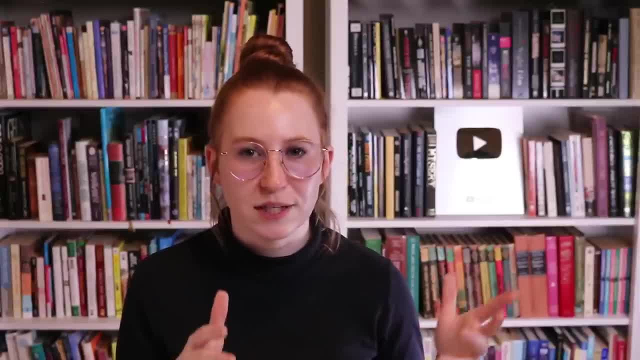 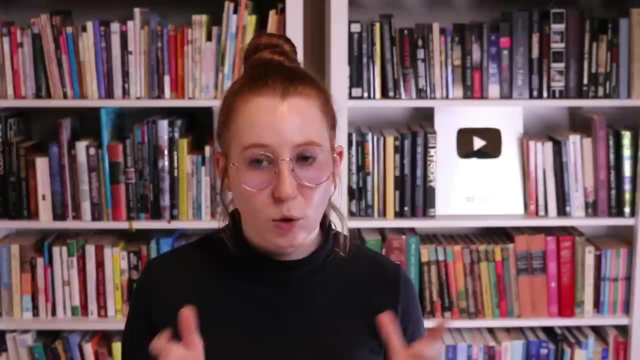 people. it's better to just use the more natural sounding sentence rather than trying to sound sophisticated or writerly. and sometimes this can happen because writers read older books more often and so that's what books sound like to them. it might also happen if you come from an academic writing. 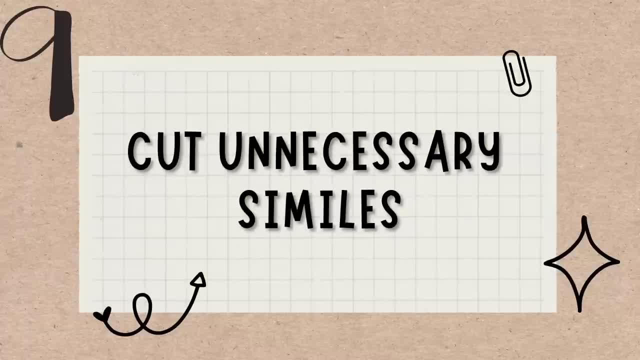 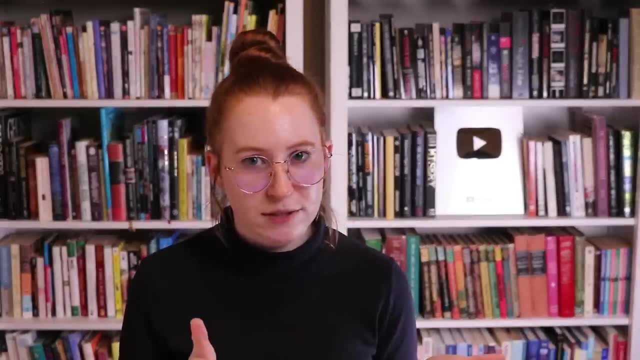 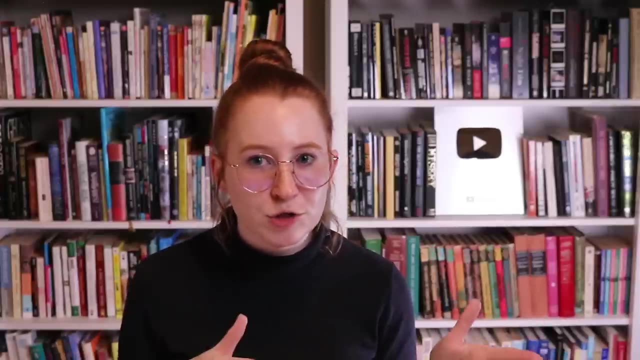 background or a scientific writing background. number nine cut unnecessary similes. so similes or comparisons using like or as do have a place in writing. i don't want to suggest that you cannot use them at all. they actually can be used very effectively, but often in amateur writing or in new. 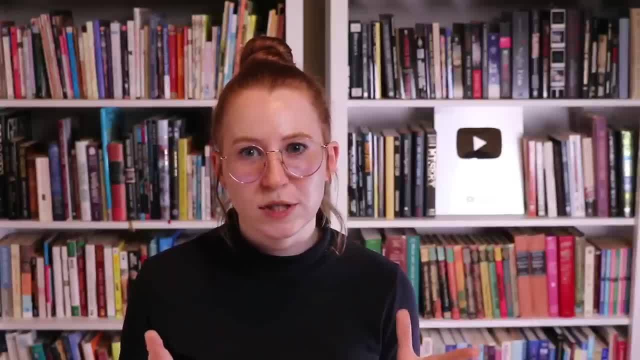 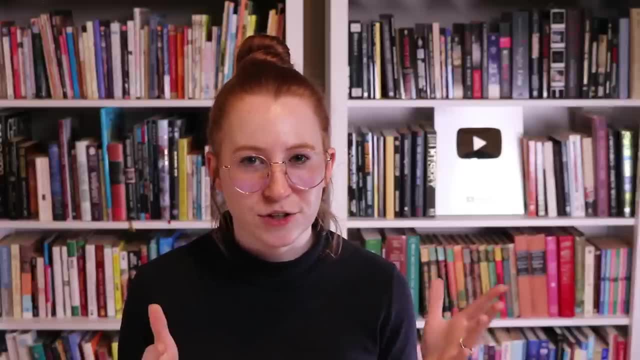 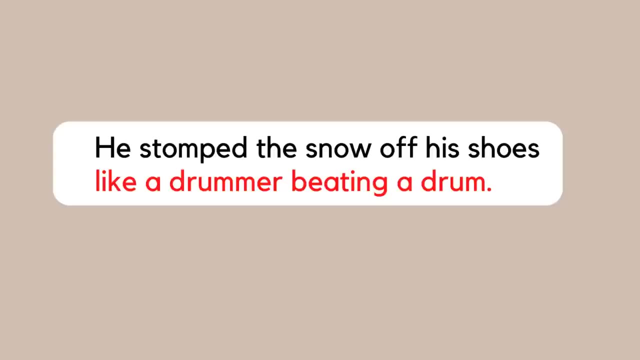 writers. they might use similes excessively or in situations where a simile just doesn't add anything sense. so normally simile is for common or well understood concepts, descriptions. things like that just don't really serve any purpose. for example, he stomped the snow off his shoes like a drummer. 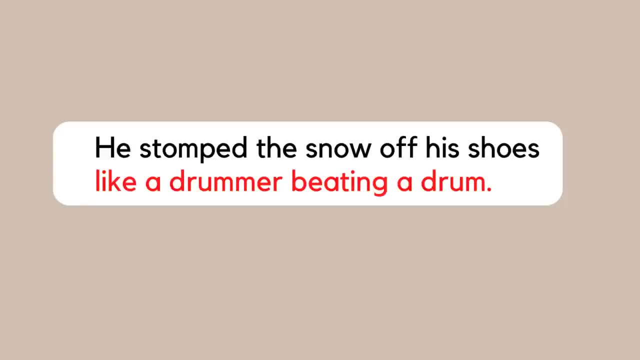 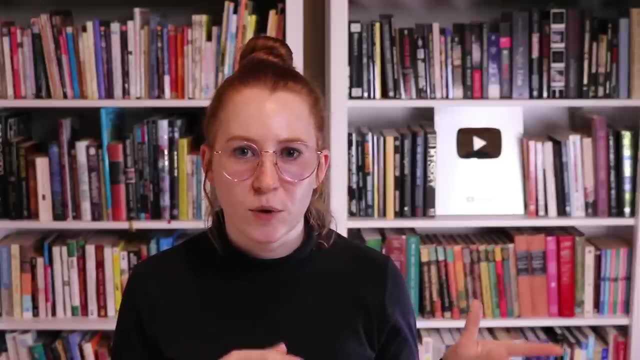 beating a drum. this doesn't really offer any meaningful additional information, because we all know what it sounds like and looks like to stomp snow from our shoes. additionally, similes don't work well when the comparison is too similar to the original thing. so with a simile, we're trying. 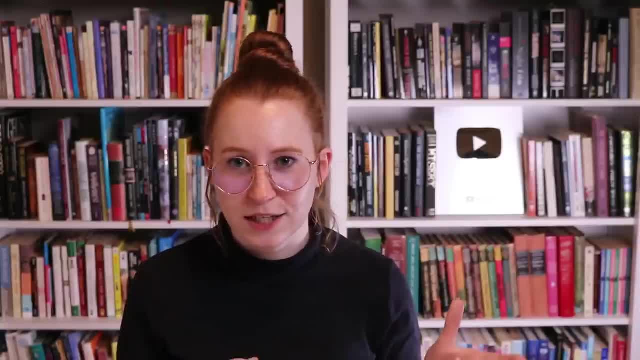 to add to or enhance the reader's understanding of what it sounds like or what it sounds like to the reader's understanding of what it sounds like or what it sounds like to the reader's understanding of the description. for example, he ran across the yard like a soccer player, running for the ball. 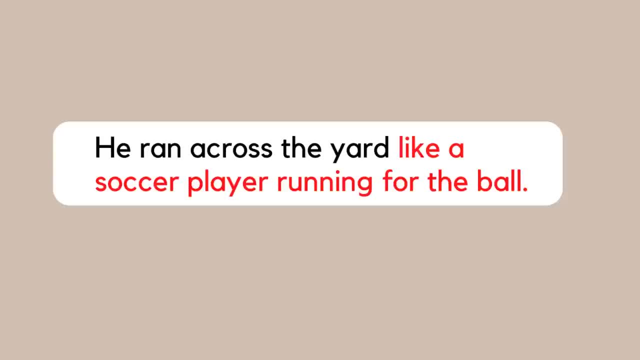 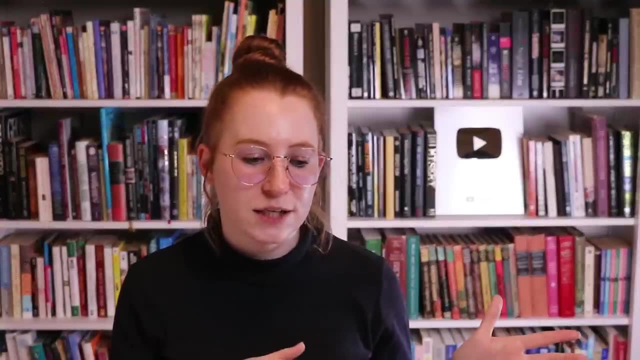 this doesn't really add new information, because it's just a different way to say that the character is running. we're not looking to just say the same thing in a different way. similes should seek to enhance the reader's understanding of something that might be unfamiliar or something difficult. 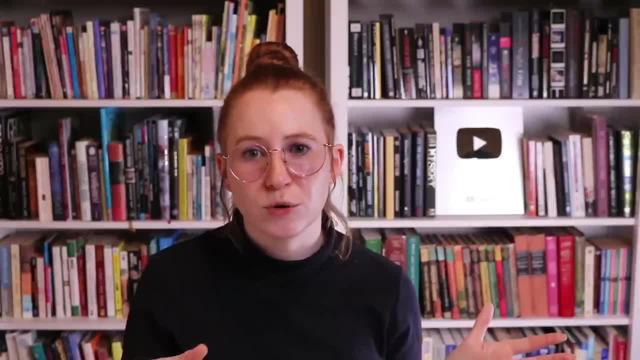 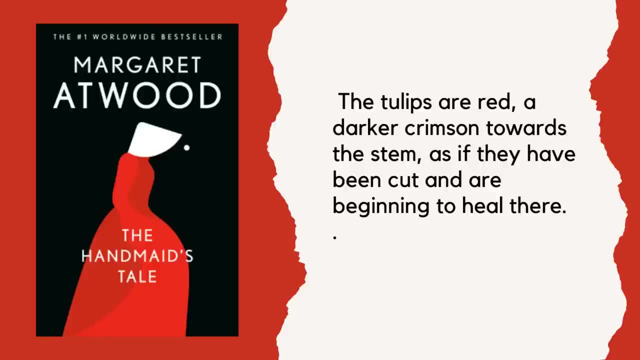 to grasp, or it should try to set the mood or the tone in a way that might not be obvious inherently, with just a simple description. for example, let's look at this simile from handmaid's tale by margaret atwood: the tulips are red, a darker crimson towards the 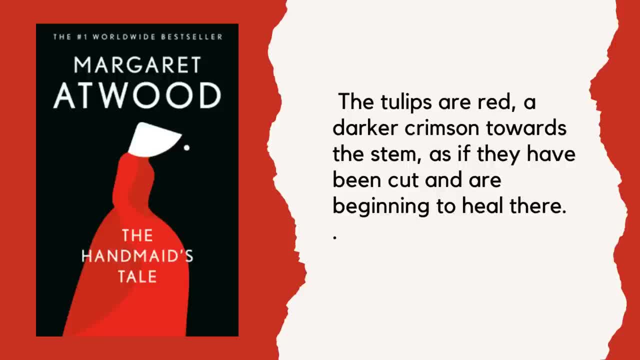 stem, as if they have been cut and are beginning to heal there. this creates a clearly dark tone, whereas just describing the tulips on their own as darker right at the stem doesn't have any particular connotation when it comes to mood or tone or vibe. here's another example. 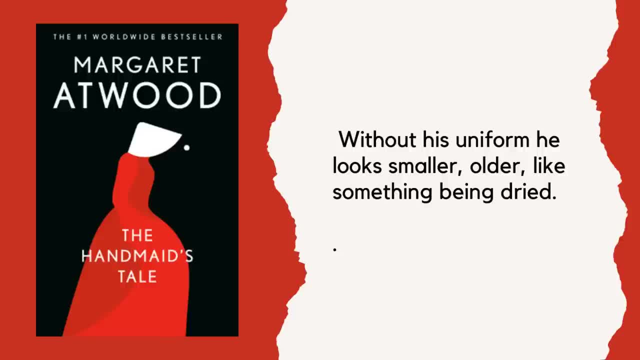 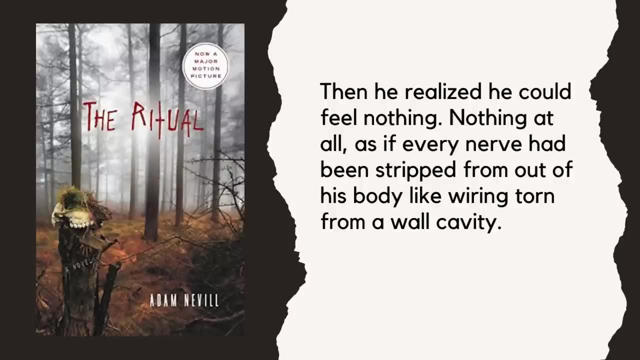 without his uniform he looks smaller, older, like something being dried. this makes the character being described feel clearly unappealing, which adds a layer of additional meaning. let's look at one last example from the ritual. then he realized he could feel nothing, nothing at all, as if every nerve had been stripped from out of his body, like wiring torn from a wall cavity. 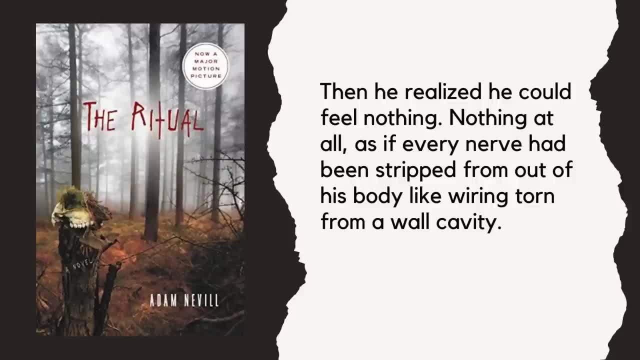 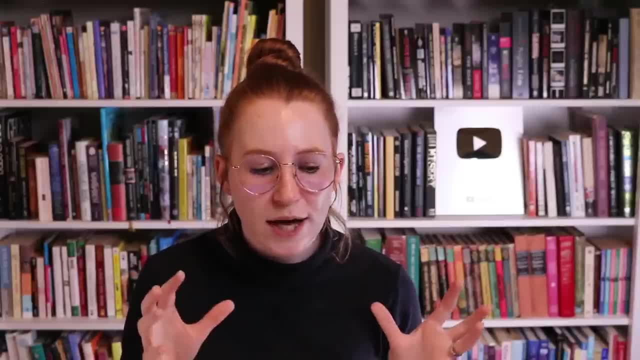 the simile emphasizes the horror element and makes the character's experience more evocative and more visceral. similes can be a great way to enhance the mood or tone or to help the reader to grasp something that's difficult to understand. just make sure that you're not including similes. 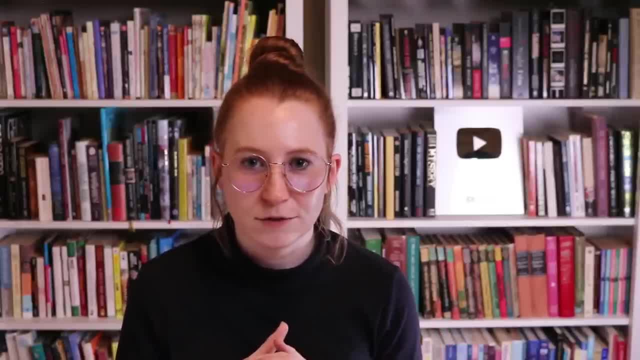 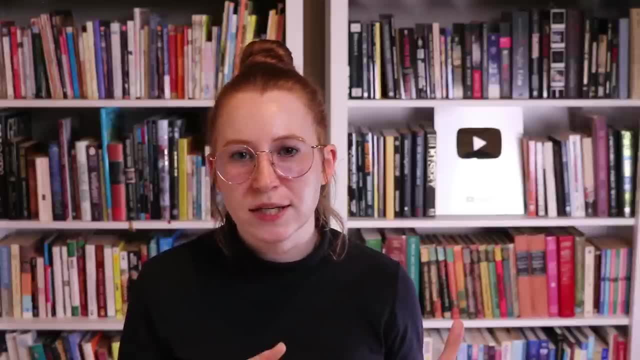 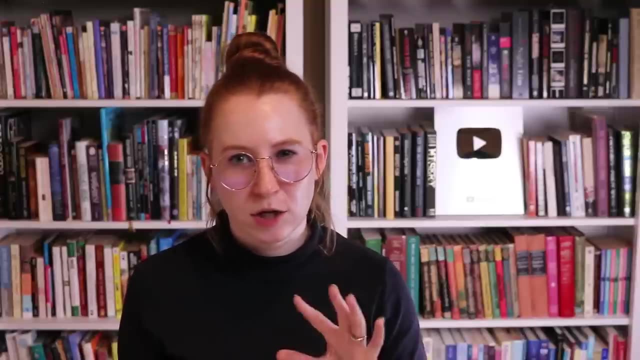 just for the heck of it, when they're not really contributing anything to the novel. number 10: use vocabulary level strategically. so vocabulary level can be a great way to convey characterization values, education level, all sorts of different things, but that's not really what i want to talk about in this video. so what i want you to focus on with vocabulary level is the 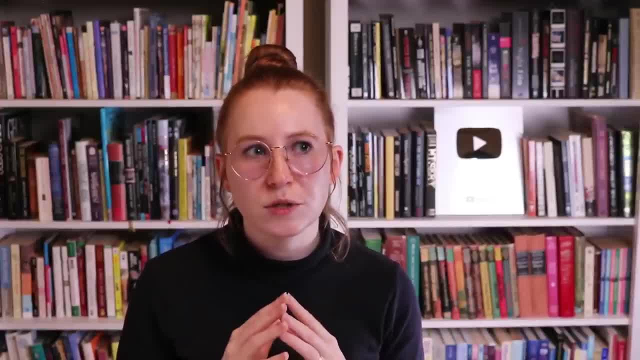 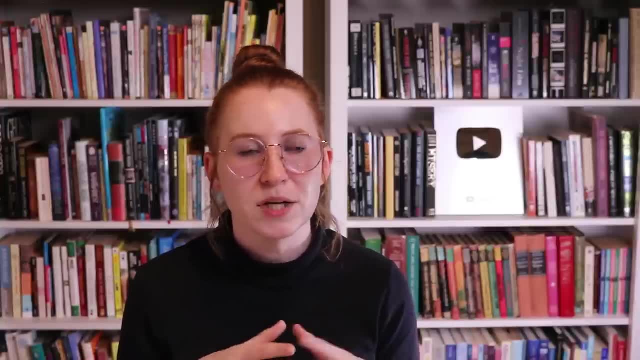 effect that it has on reading speed. so when you use more advanced vocabulary, bigger words, even if you use bigger words that are fairly common, not super obscure, it really is a great way to slow down the reader. this isn't necessarily a bad thing, it's just something to be aware of some. 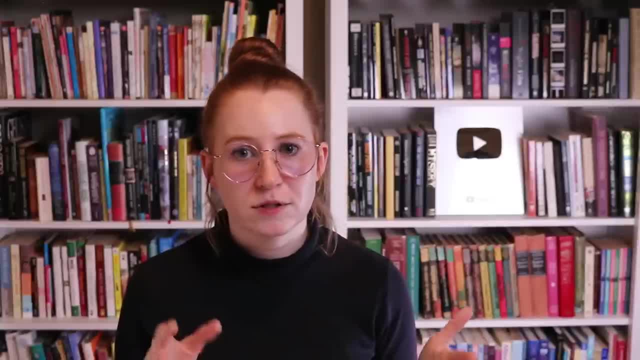 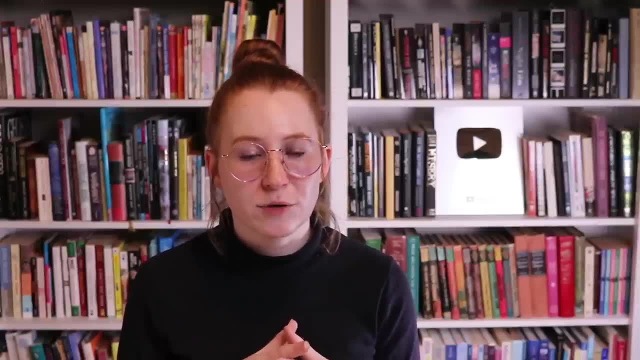 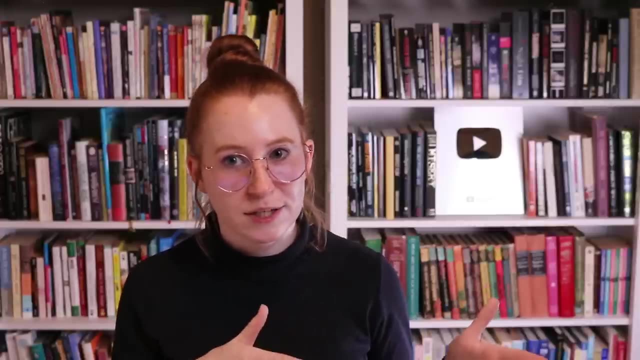 books are meant to be read more slowly. some genres, some target reader groups like to read things slowly, whereas other groups prefer something faster paced. other genres do better with a faster, more clipped pacing, which can be better achieved with a lower vocabulary level. so pay attention to how your word choice is in terms of complexity of the words, advancedness of 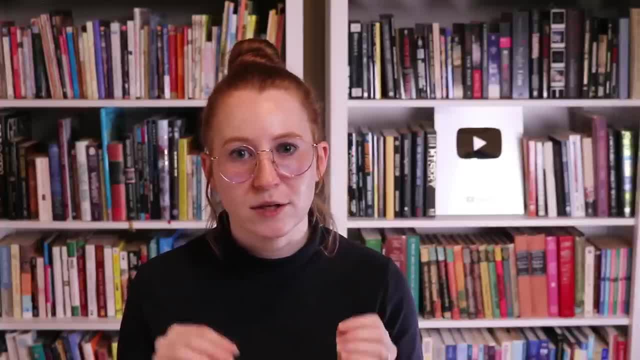 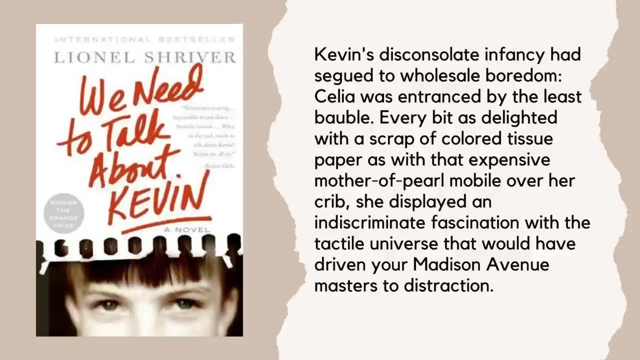 the words can impact how slowly or quickly the reader gets through the text. let's look at an example from we need to talk about kevin. this is a good example of more advanced vocabulary being used to convey character in a novel, but also in my opinion, this book is best read slowly and the 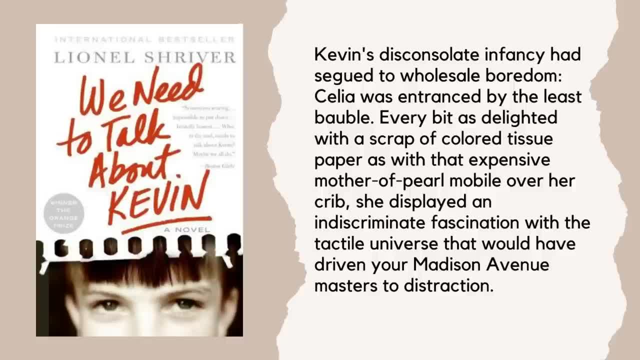 more advanced vocabulary helps to slow the reader down and really experience the story alongside the protagonist. so in this excerpt the protagonist is describing the difference between her troubled son kevin and her daughter c� sheep. and then the Reg poster. she's not reading the original poblanitary event with wantedUh and uh, like edward, come on, i'm. 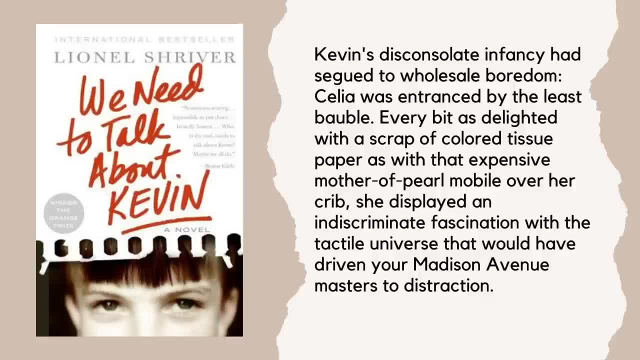 Celia's infancies. Kevin's disconsolate infancy had segued to wholesale boredom. Celia was entranced by the least bauble. Every bit as delighted with a scrap of colored tissue paper is with that expensive Mother of Pearl mobile. over her crib She displayed an indiscriminate 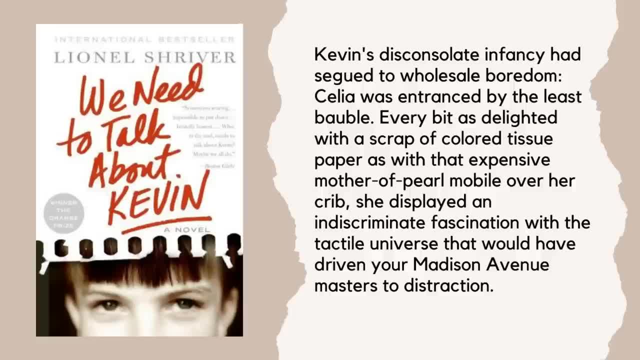 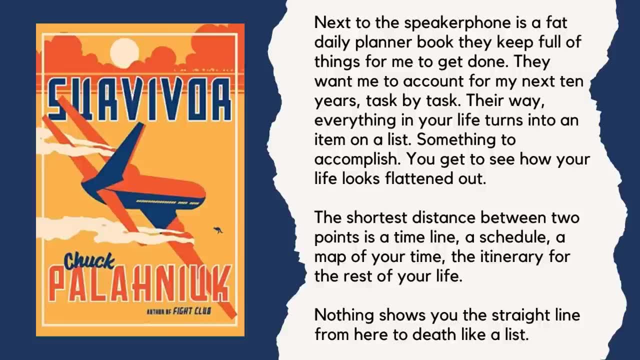 fascination with a tactile universe that would have driven your Madison Avenue masters to distraction. We can compare this to a book that, again, in my opinion, is a bit of a quicker read, yet with no less personality or characterization in the writing. This is an excerpt from Survivor. 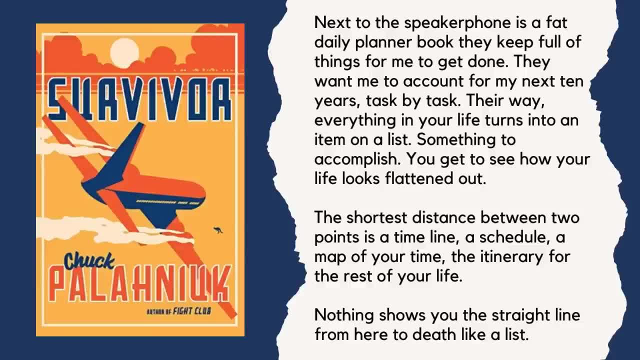 by Chuck Palahniuk. From this example we can really tell that a simpler vocabulary level doesn't mean that you can't make interesting points or have a unique style. Next to the speakerphone is a fat daily planner book. they keep full of things for me to get done. They want me to. 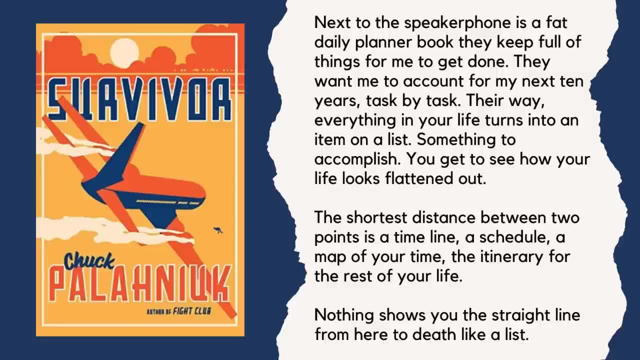 account for the next 10 years, task by task. Their way, everything in your life turns into an item on a list, something to accomplish. You get to see how your life looks flat. You get to see how your life looks flat. You get to see how your life looks flat. You get to. 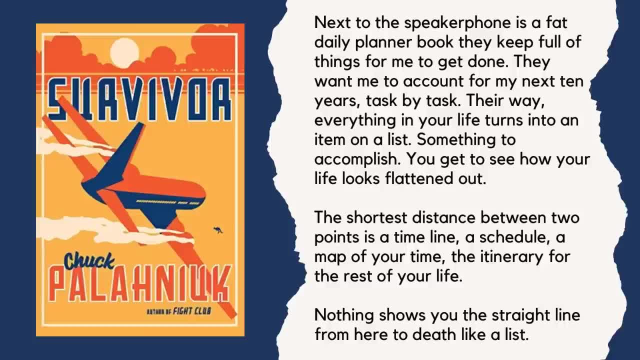 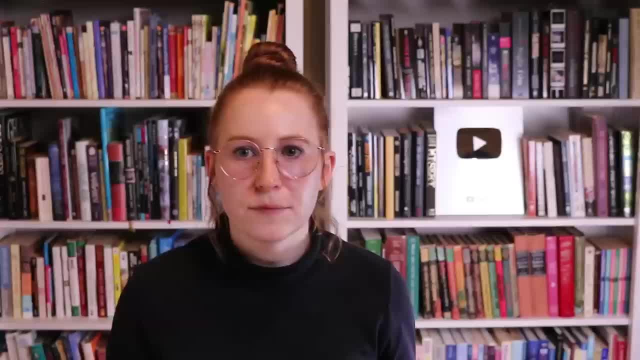 flattened out. The shortest distance between two points is a timeline, a schedule, a map of your time, the itinerary for the rest of your life. Nothing shows you the straight line from here to death like a list. So that excerpt from Survivor is written on a third grade level and the excerpt 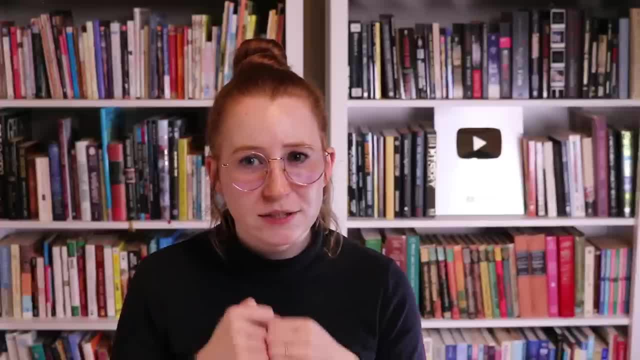 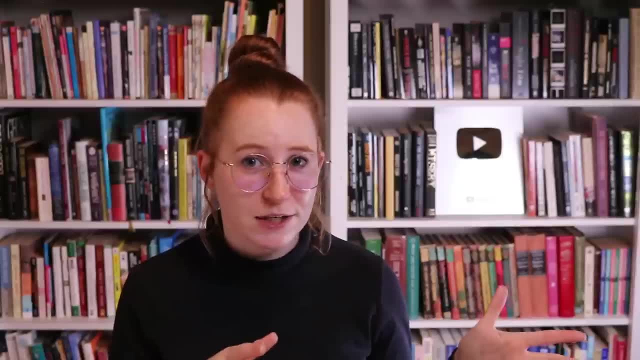 from We Need to Talk About. Kevin is written on a ninth grade level. This is a really big difference in reading level. but both books feel mature, They both feel interesting, They both have a lot of characterization. so there's not any sense that it's less sophisticated to write a book like this. 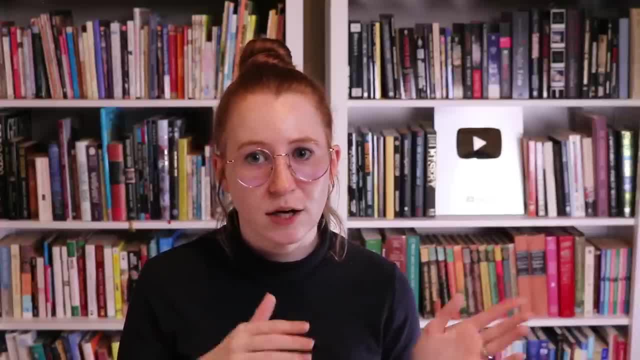 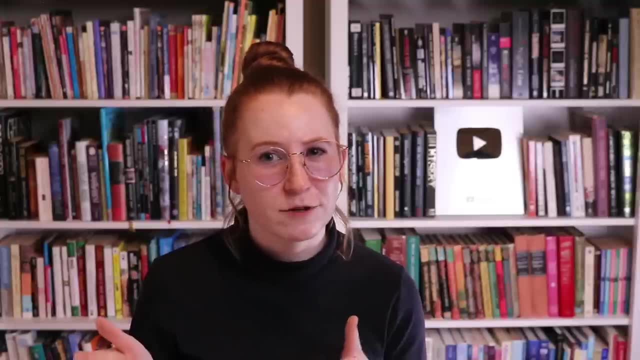 At a lower reading level. what it does do is it makes the book read a lot faster, I think. for me, I read Survivor in probably two or three days, whereas I read We Need to Talk About Kevin over probably a month, a month and a half. It just was a book that, in my opinion, felt like it needed to. 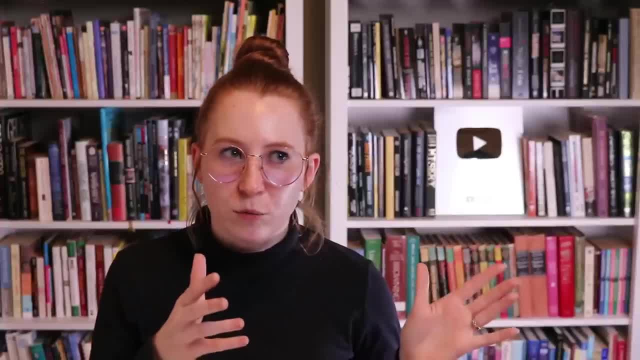 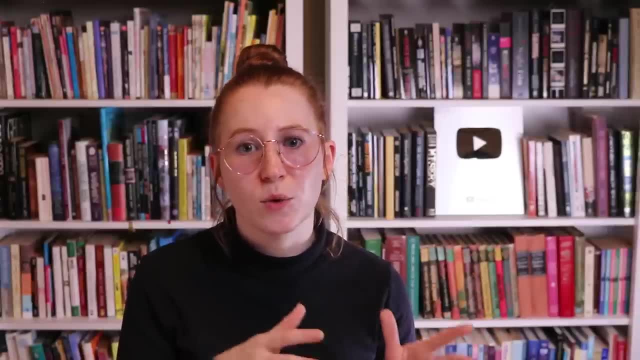 be read more slowly. Think about the vocabulary words you're choosing and how it's impacting the pacing of your book. Think about the story and what it calls for, how quickly you want it to be read, how quickly it should be read. The vocabulary level will guide the reader on how long to spend reading the book. 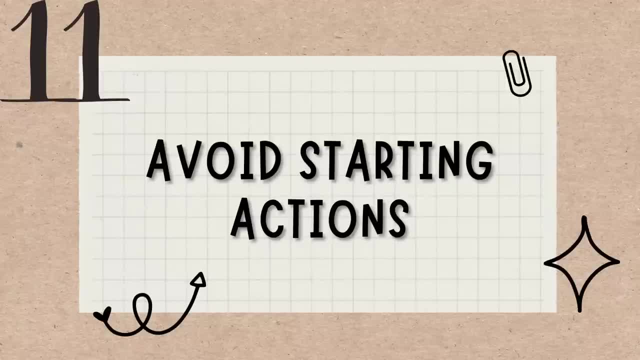 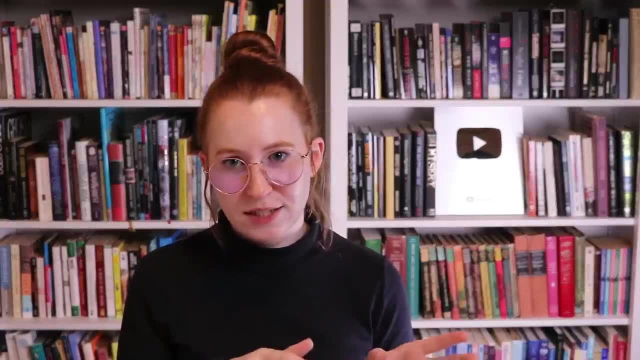 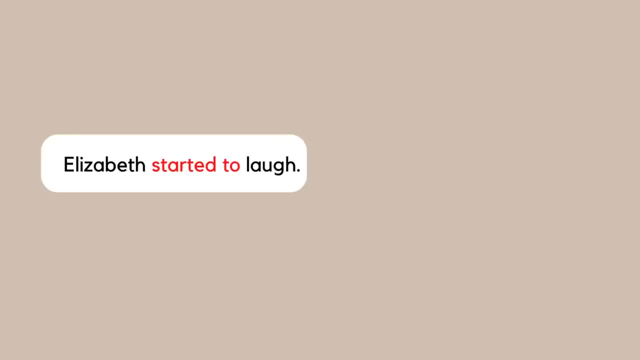 Number 11, avoid starting actions. This is another super, super easy one. Having characters start or begin actions reduces the immediacy of the action and almost never enhances understanding. For example, Elizabeth started to laugh and Elizabeth laughed will convey the same meaning in the vast 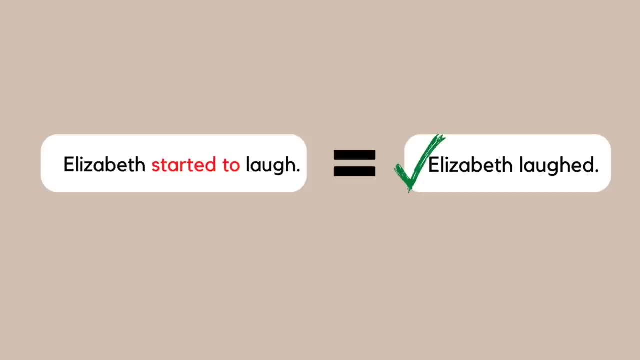 majority of circumstances. but Elizabeth laughed, feels much stronger and more immediate. For the same reason, Elizabeth laughed and Elizabeth laughed. Elizabeth laughed and Elizabeth laughed for the same reasons. Mark lunged forward and punched John is stronger than Mark lunged forward and began to punch John Again. if you have a situation where it does change the meaning to 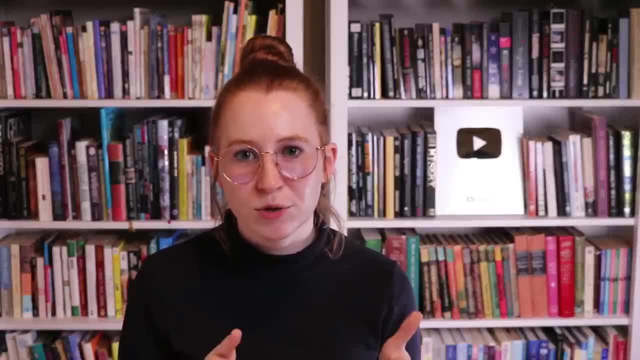 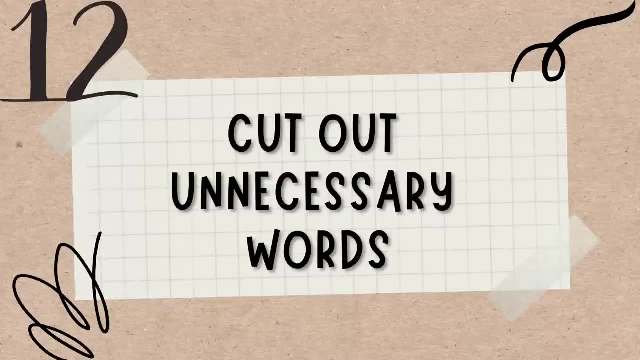 you start or began, then by all means do so, But in the majority of cases this can just be a bad habit that writers get into, and cutting out start and began from your writing will make it stronger. Number 12, cut out unnecessary words. Wordiness can, of course, be a stylistic choice. 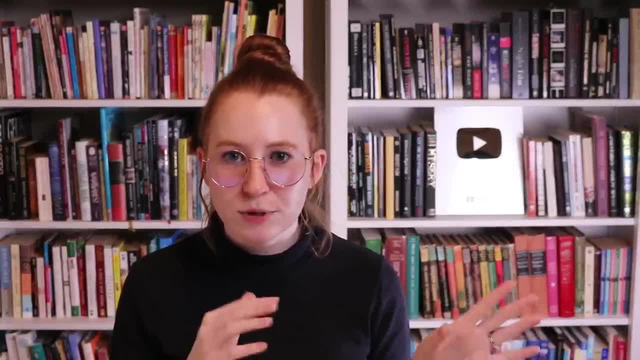 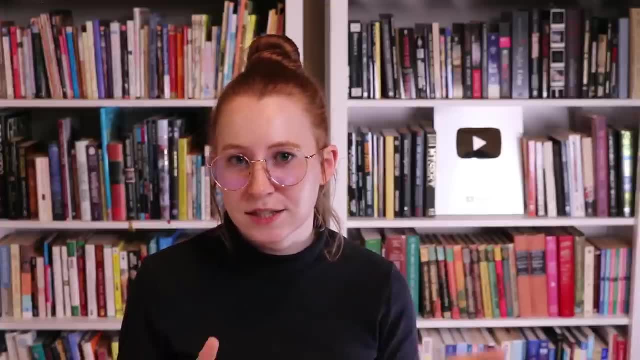 but I'm not really talking about wordiness as a style choice here, But rather just using an excessive amount of words that don't add or enhance meaning. So this can create unnecessary distance from the action and it can also bury the point that you're trying to make. 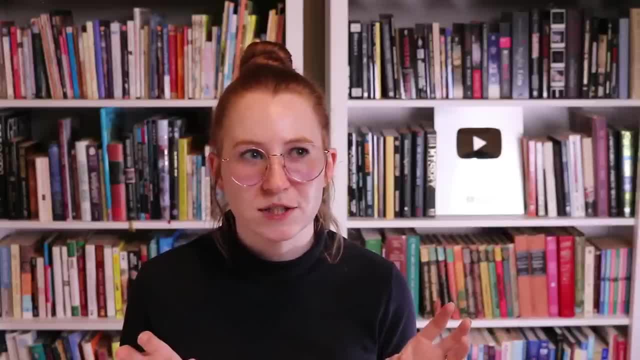 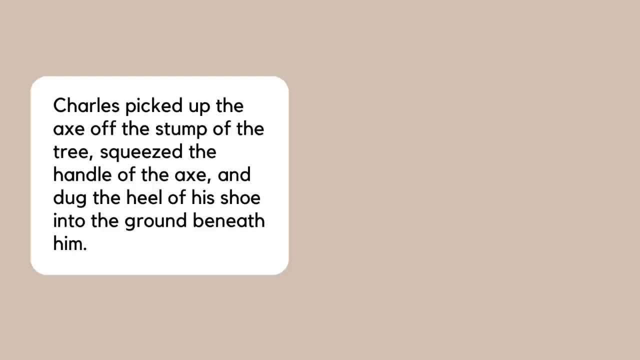 or just create a sort of cluttered sense to your writing, where it just doesn't feel crisp and clean. Let's look at this example, which depicts very clearly a common reason for overriding, which is constantly describing something as being of something else. Charles picked up the axe off the stump of the tree, squeezed the 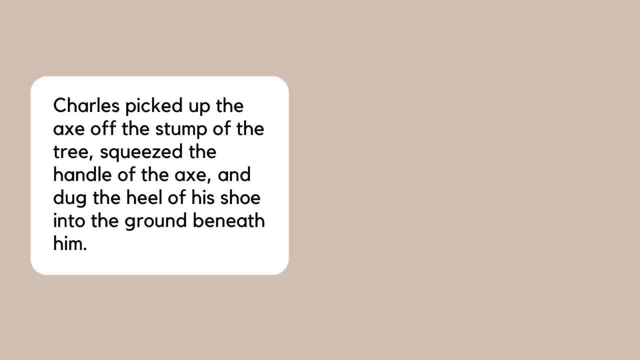 handle of the axe and dug the heel of his shoe into the ground beneath him. This could easily be cut down to. Charles picked up the axe from the stump, squeezed the handle and dug his heel into the ground. We don't need stump of the tree because 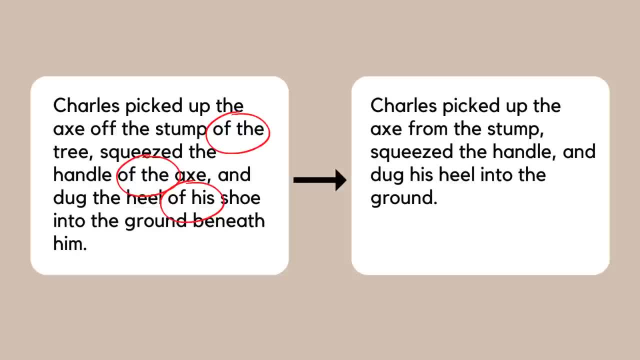 we know the stump is from a tree. We don't need heel of his shoe, because we can assume Charles is wearing shoes. We don't need handle of the axe, because we know this is talking about the axe, Besides of being a common indicator of extra words. 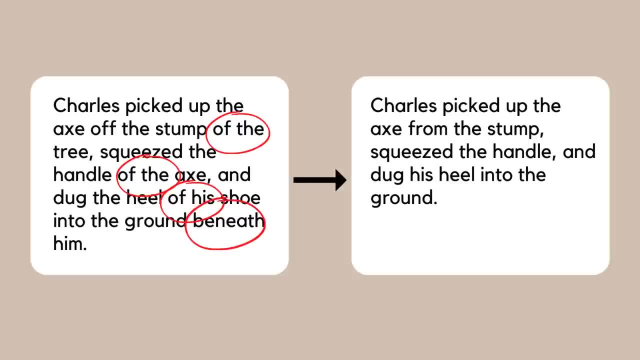 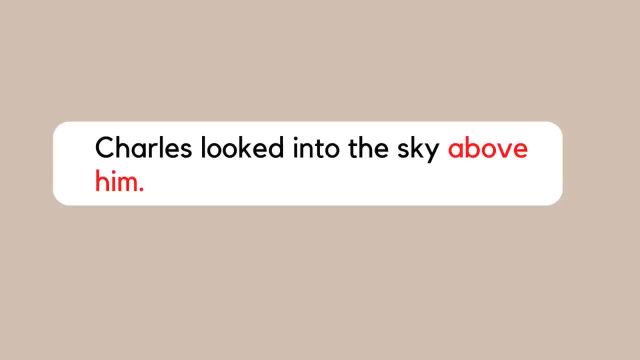 the ground beneath him is also unnecessary. We already know the ground is beneath him. Unnecessary directional or location-based descriptions can also really blow writing. For example, if we were to write something like Charles looked into the sky above him. we already know the sky is above him, so it's an unnecessary amount of extra words. 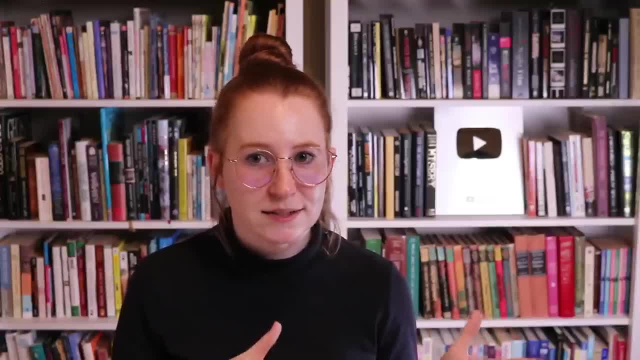 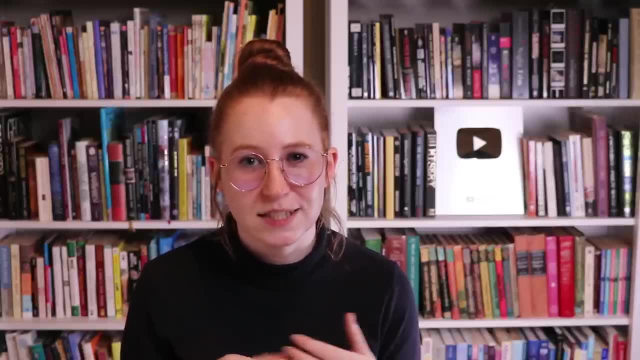 This might not sound like a huge deal and in isolation it really isn't a big deal, but over the course of an entire novel this can add up to tons and tons of extra words that just create a lot of distance and clutteredness in the writing. 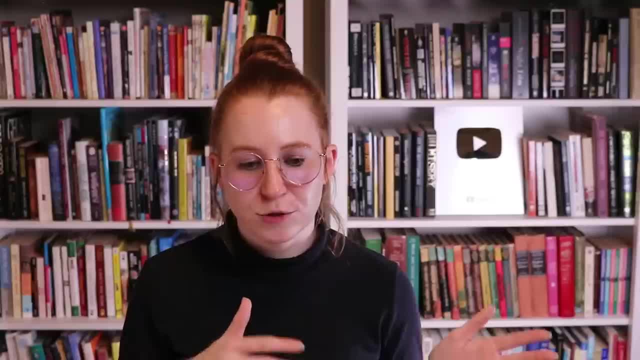 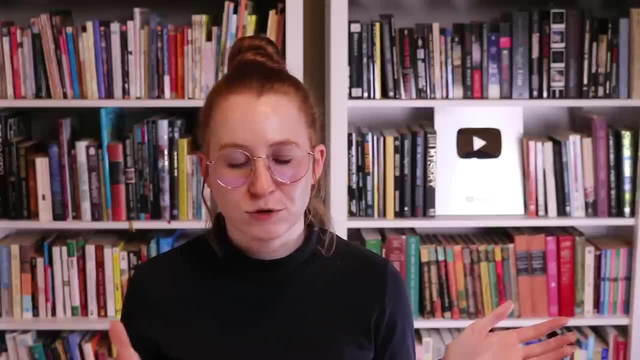 Keep in mind, though, that sometimes you might use extra words either to control the flow or pacing of a sentence to make it sound better, or we might add extra words when there's a detail that we want to include. So, for example, we might want to describe Charles' shoe in this excerpt. 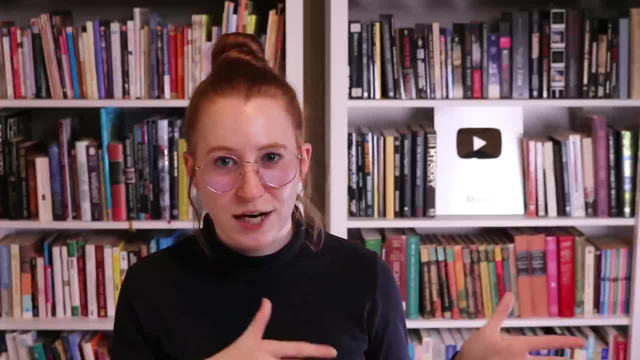 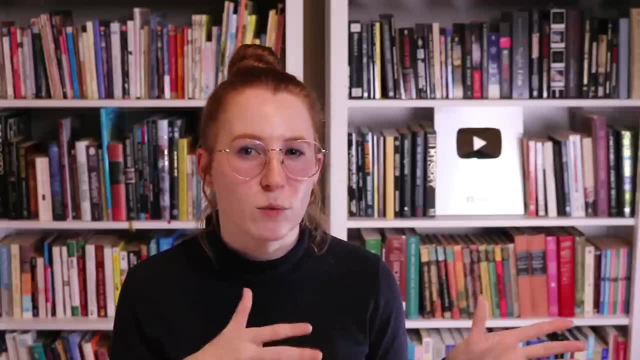 So in that case we might say he dug the heel of his boot into the ground because we want to make sure that the reader knows that he's wearing boots rather than just regular shoes. So there may be reasons why you want to do this, but often these are good signs that 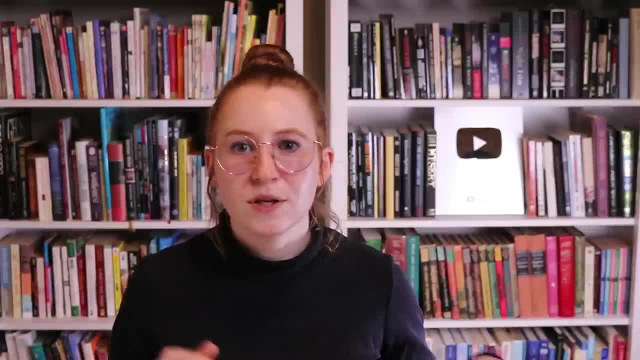 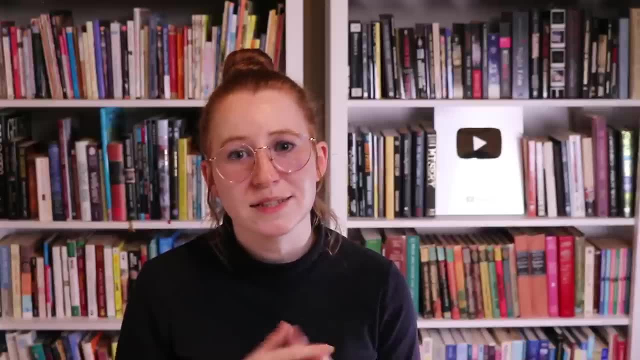 there's just a lot of unnecessary words that could be cut down, So that is all I have for you guys to do today. I really hope you found this video helpful. If you have any tips that have helped you to write better sentences, please leave them in the comments. If you want to help support the 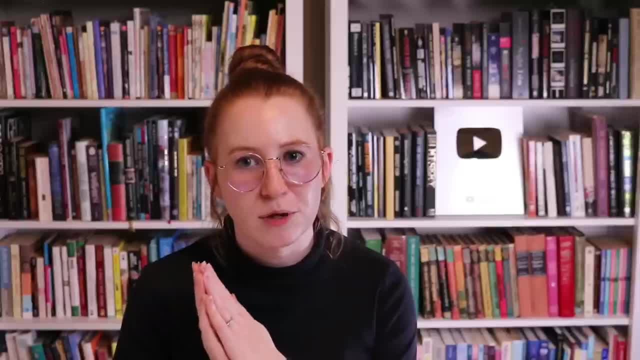 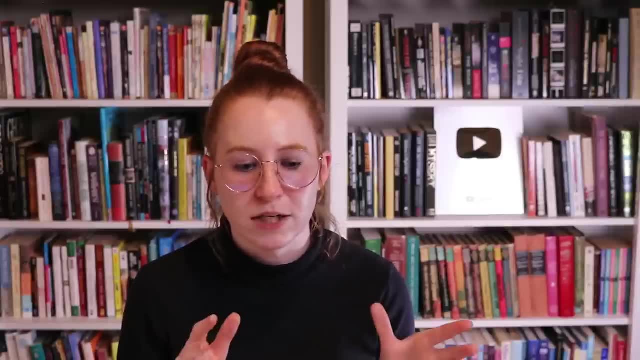 channel. I do have a Patreon. We now have a Discord server available at the $2 tier and at the $5 and up tier. there is some supplemental things to go along with the video. So, for example, a cheat sheet will go up for this video and also there are some Q&A videos.